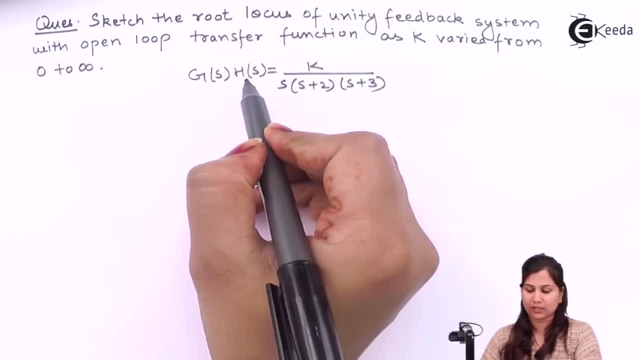 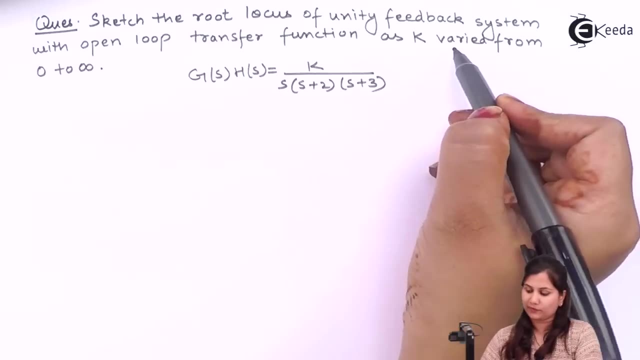 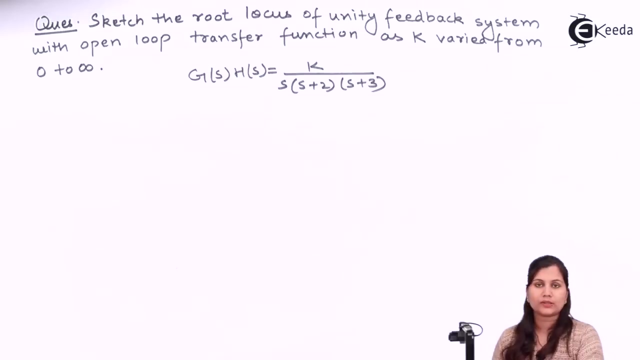 transfer function given to us as gs. hs equals to k upon s s plus 2, s plus 3, as the value of k is varied from 0 to 1. to infinity. So let us sketch the or plot the root locus of this system. We will follow. 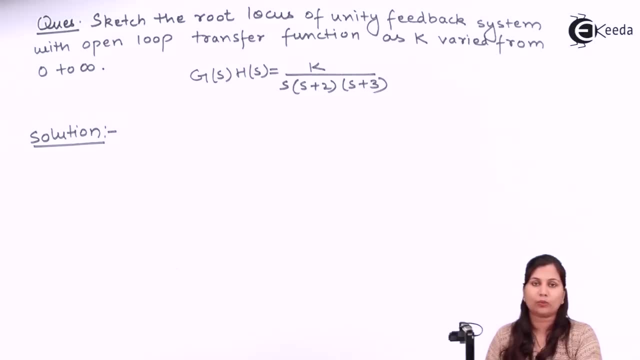 the rules or the steps of the root locus technique, one by one, to plot this root locus. The first step is to determine all the poles and zeros of this system. So, as you see, here we have the poles and zeros of this system. So, as you see, here we have the poles and zeros of this system. So, as you see, here we have. 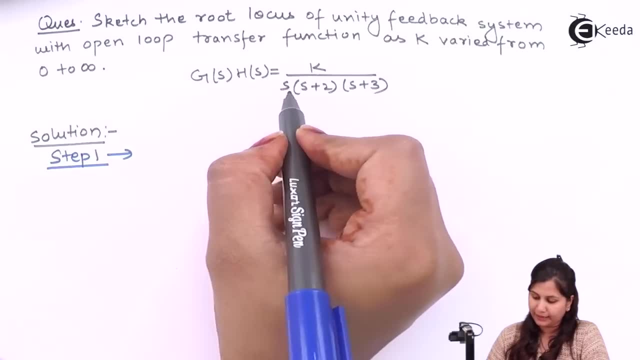 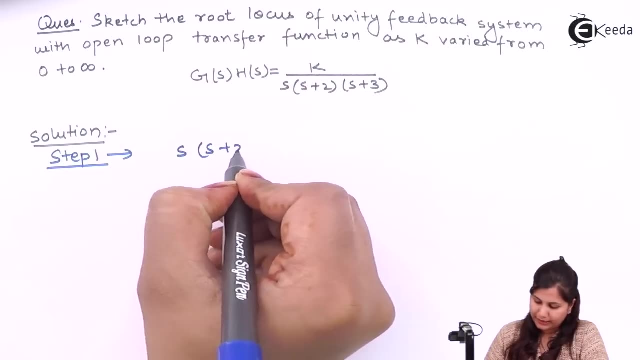 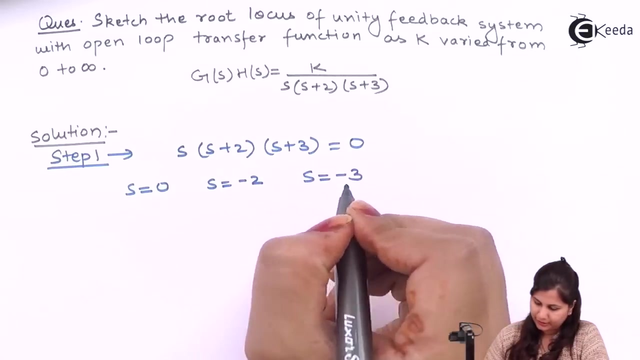 that the poles. they are obtained by equating this denominator term to 0. So s s plus 2, s plus 3 equals to 0.. So we have the roots of this equation. as s equals to 0, s equals to minus 2 and s equals to minus 3, at k equals to 0.. 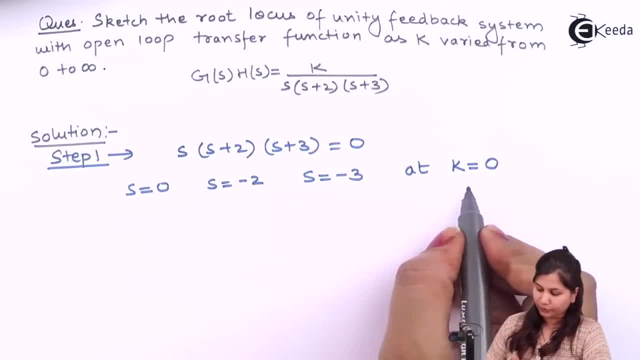 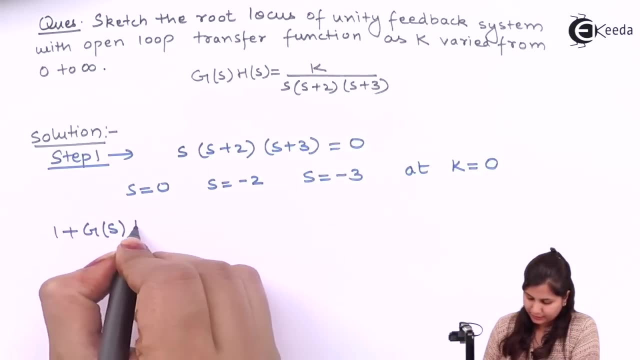 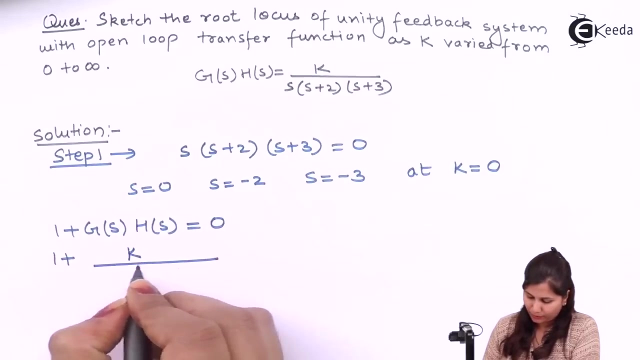 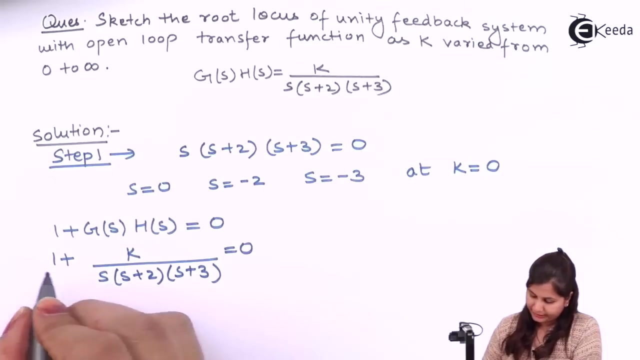 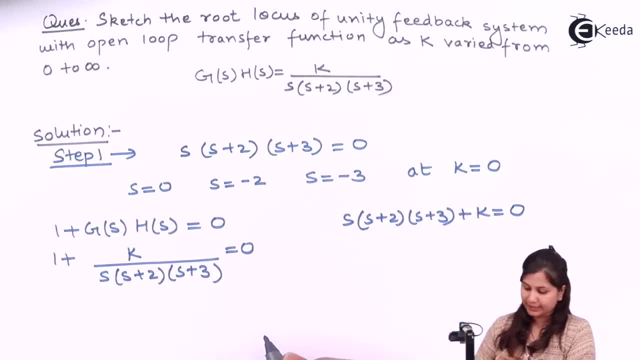 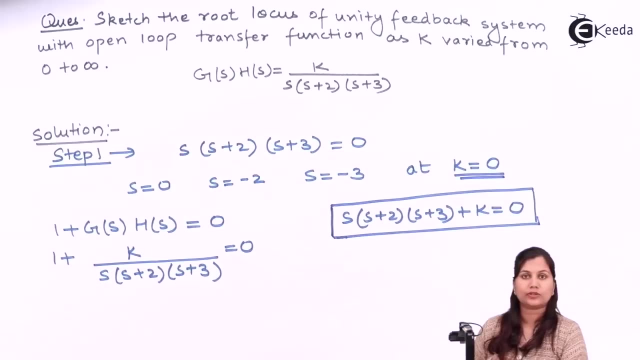 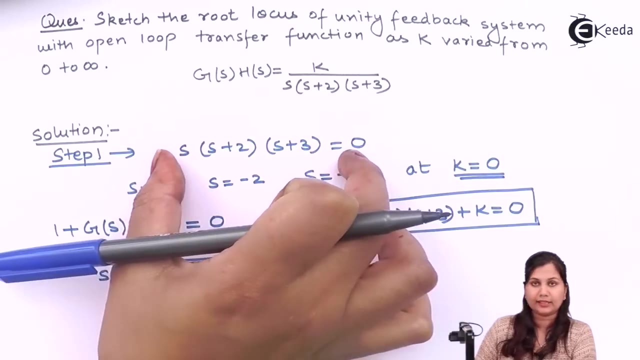 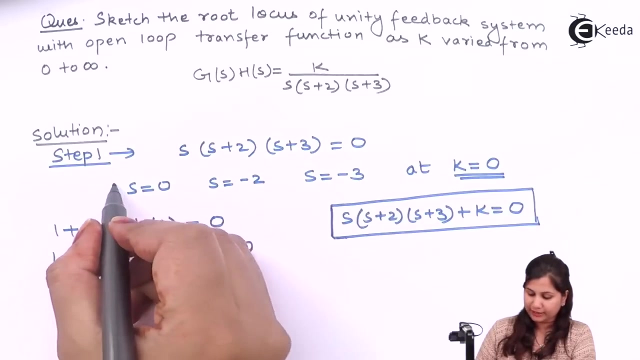 plus k equals to 0. This is our characteristic equation of this system. Now here we are. taking the value: k equals to 0. So if k is equals to 0, this remaining term will be equal to 0. So this is here. Now take the values. take out the values roots of this equation. we are getting 3 roots. 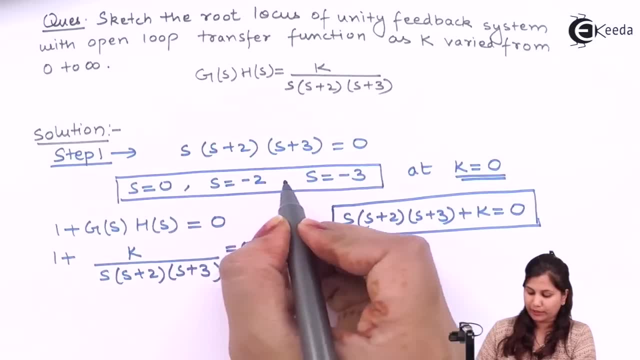 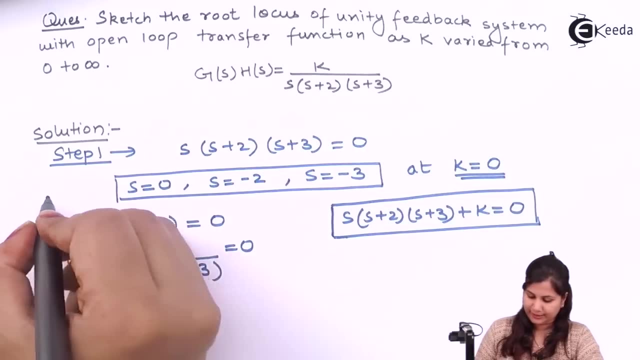 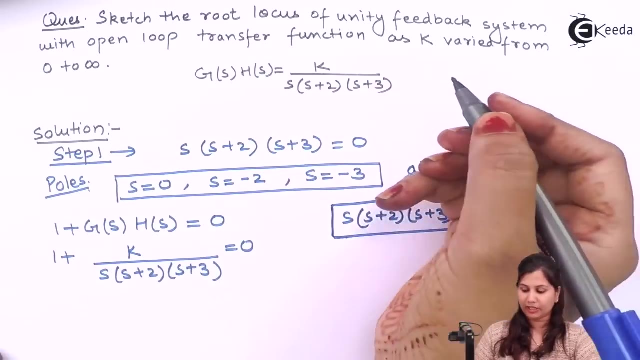 s equals to 0, s equals to minus 2 and s equals to minus 3.. So these three values, they are the poles of this system. Okay, and 0, because here we are not having any 0. So these poles, the root. 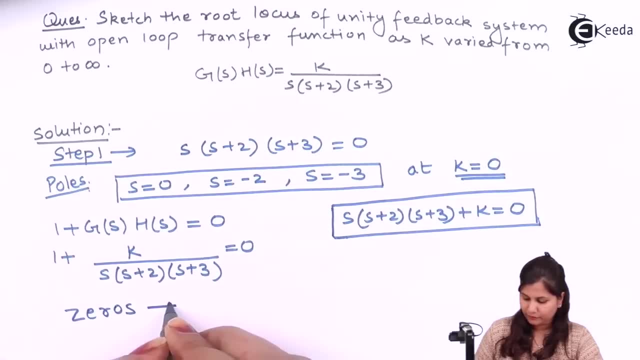 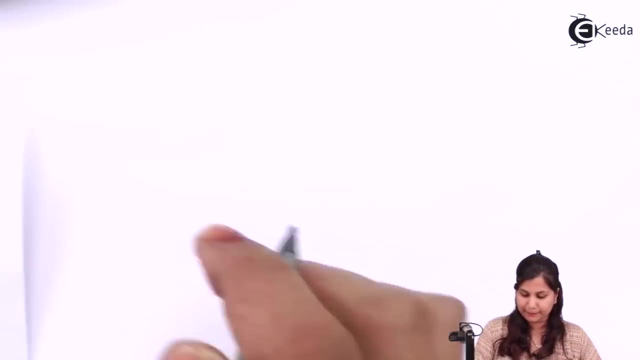 locus. we are having no 0 for this system. Okay, so in the first step we have obtained the open loop poles and zeros of this system. Now, second step is the starting and the ending point of the root locus. Starting the root locus, they starts from the poles and they terminate. 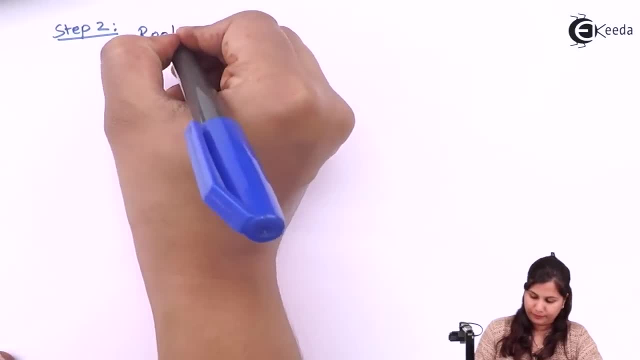 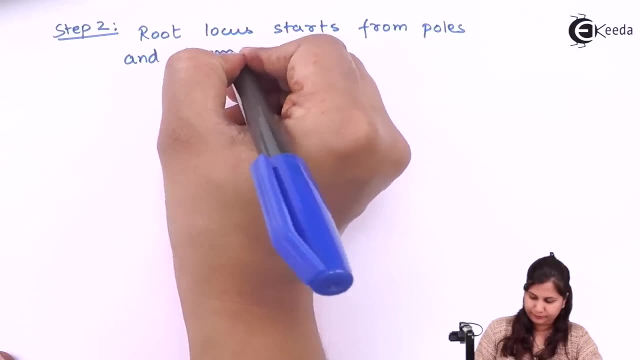 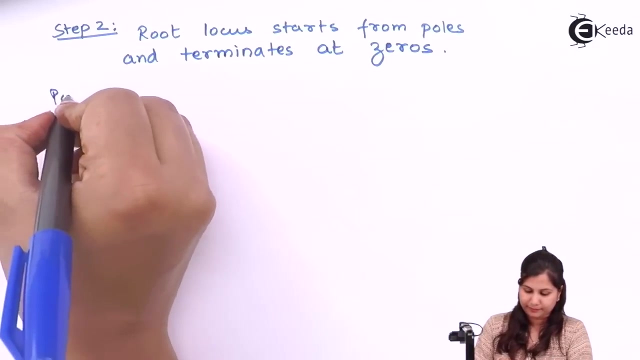 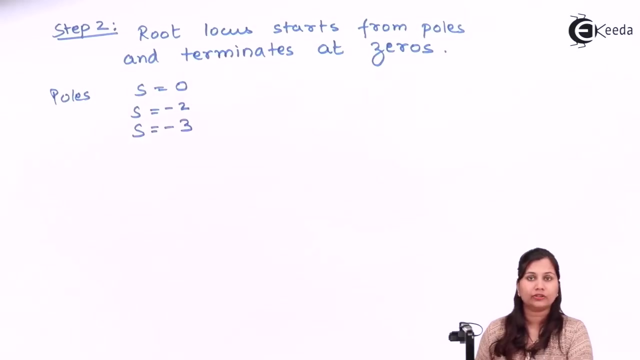 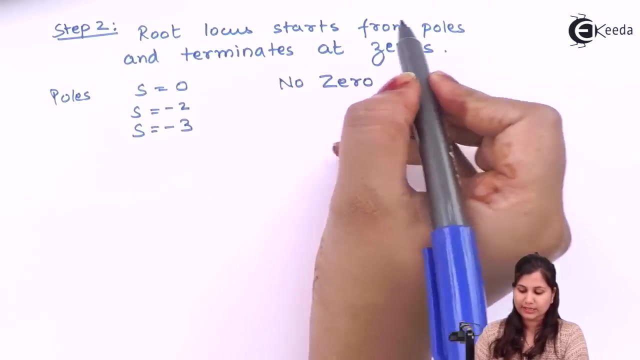 at the zeros. Here we are having three poles: s equals to 0, s equals to minus 2 and s equals to minus 3, and zeros. we are not having any 0. So for this system we have obtained the open, the root locus. it will start from the pole, but it will terminate here at infinity. 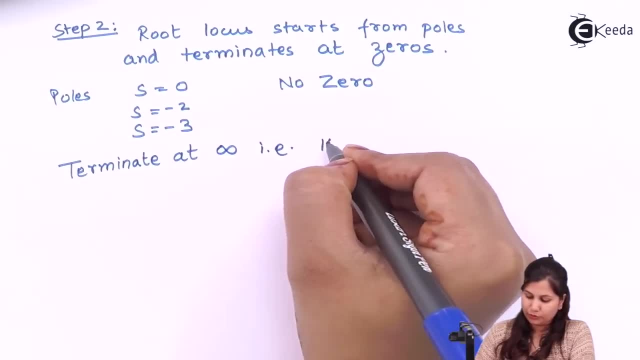 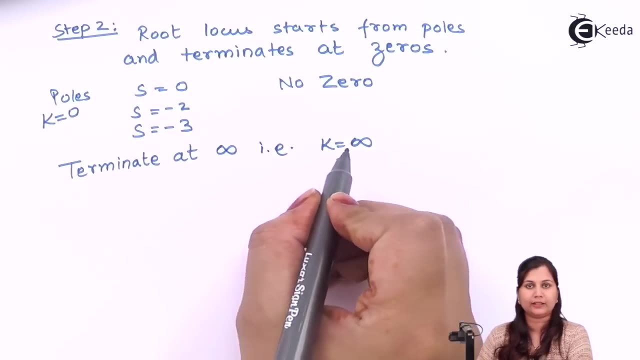 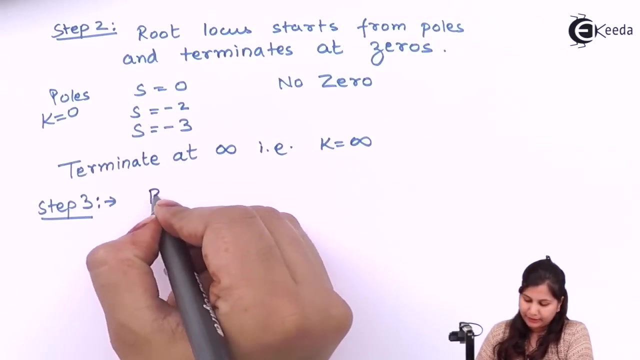 Okay, that is k equals to infinity. It will start from k equals to 0 and it will terminate at k equals to infinity. So this is the starting and the ending point of the root locus. Now we are going to determine the direction of the root locus branches. Here we are having p greater. 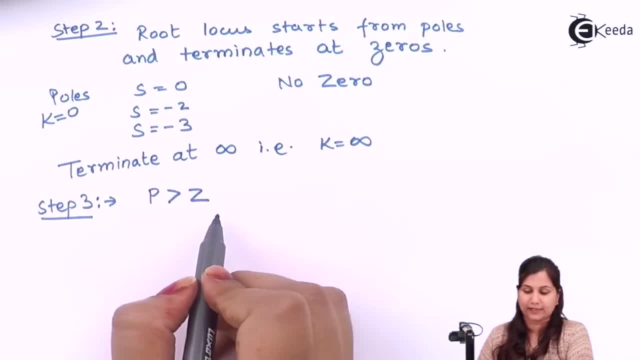 than z, that is, the number of poles is greater than 0.. Poles are 3 and 3 is greater than 0. So the number of branches will be that equals to number of poles. that is, there will be three branches. Okay. 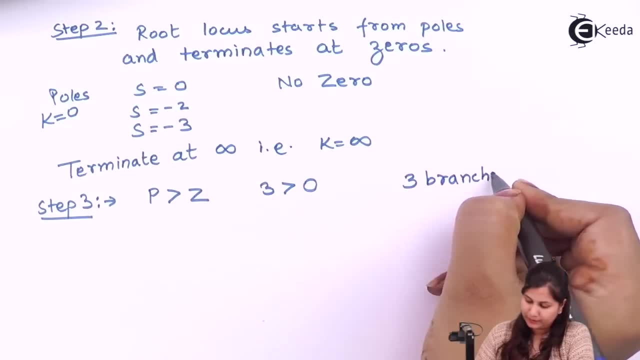 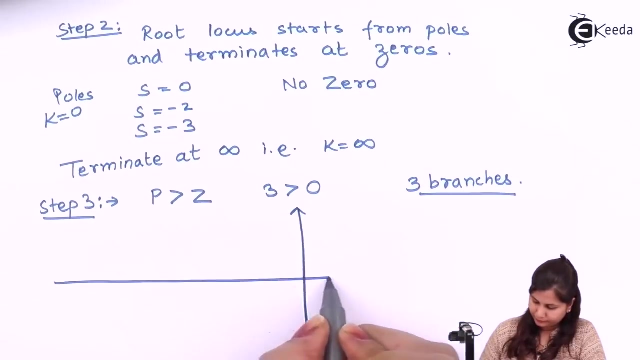 Three branches of root locus. Now plot these roots, or the poles of the system, on the s plane. This is our imaginary axis. This is real axis. Okay, This is 0, s equals to 0. Then we have minus 1, minus 2, minus 3 minus 4.. 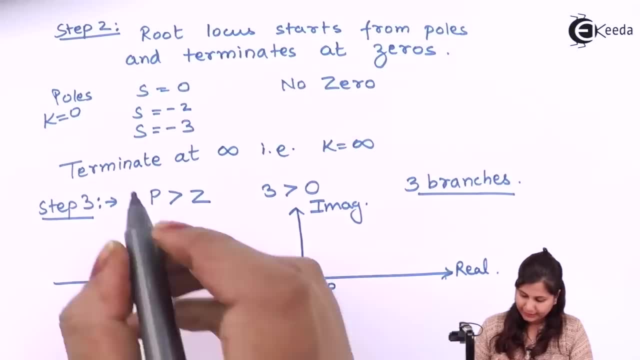 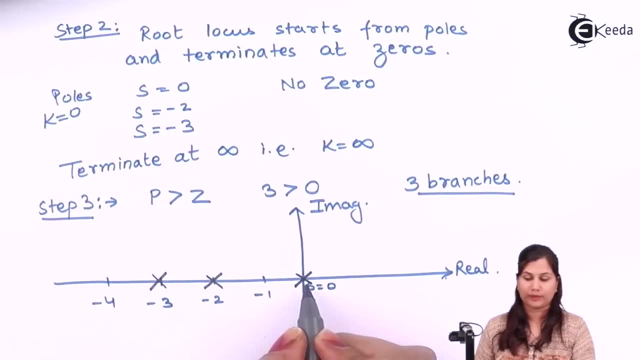 Now, s equals to 0 is a pole, S equals to minus 2 is a pole, and s equals to minus 3 is a pole. So we are having three poles now to determine the direction of the root locus branches. take three points. Take point across 3.. 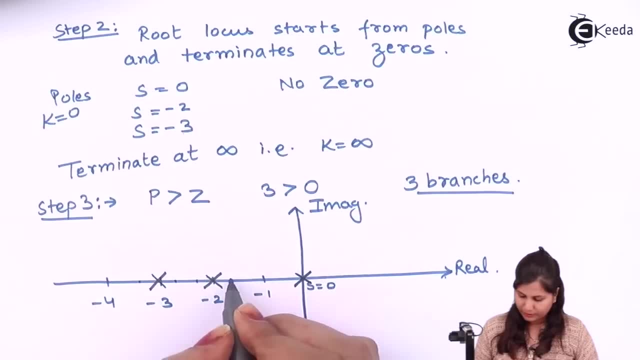 Take point across. 2. Take point across. 3. across all these three poles. suppose this is p1 and for this pole this, there are two points p2 of about this second pole, and there are two points across this pole also. so if we start from here, from this point, then calculate the number of poles and zeros on the right. 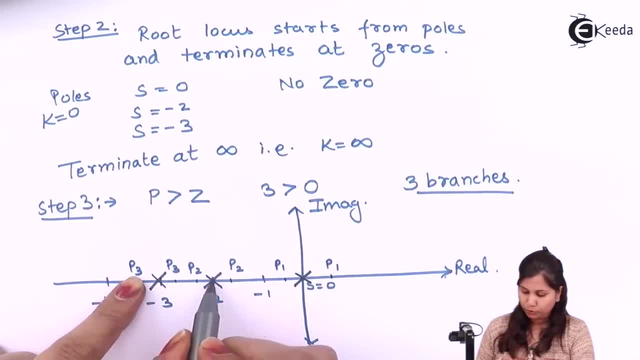 hand side of this point. we have one, two, three, three poles on the right hand side of this point, so the direction of the root locus for this pole s equals to minus three. it will be towards this point. okay, so it will be in this direction. now for this point. p3, the number. 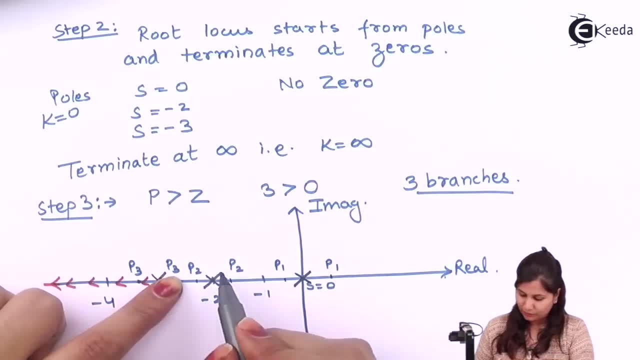 number of poles and zeros on the right hand side is 1, 2. that is, even So, the direction of root locus. for this pole s equals to minus 3. it will not be in this direction, that is, towards this point. Now for check. for this pole s equals to minus 2.. For s equals to minus 2. we have taken 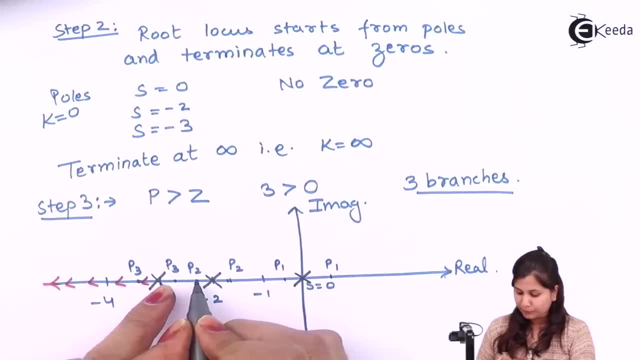 two points. First, check for this point. For this point we are having the number of poles as 2 on the right hand side, So the direction of root loci will not be towards this point. Now for this p2 point, the number of poles is 1 on the right hand side, So the direction of root loci will be 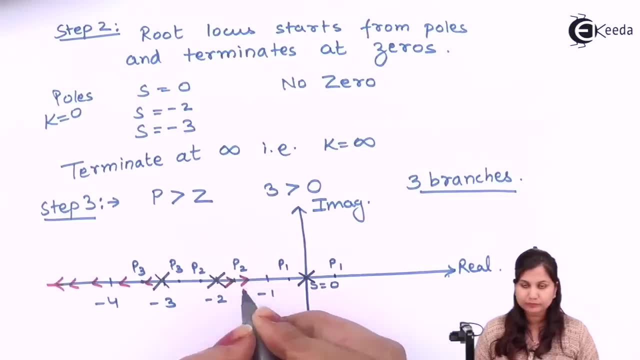 towards this point. Now for p1, the number of poles is 1 on the right hand side. it is odd, so the direction of root loci will be towards this point. okay, and for this point the number of root loci is the number of poles is 0 on the right hand side, so it will not be in this direction. 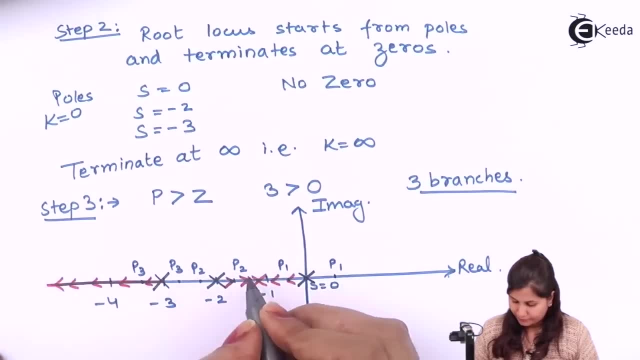 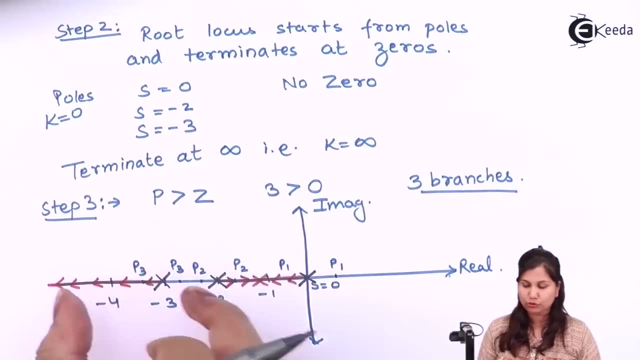 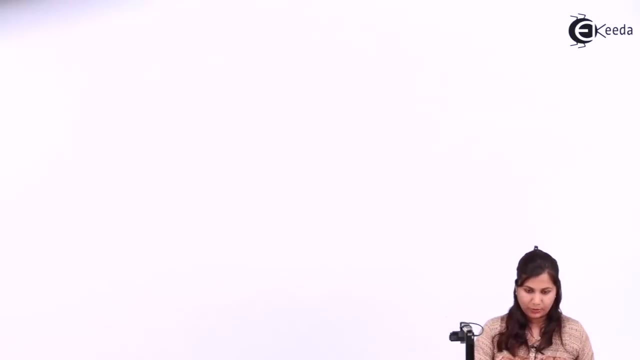 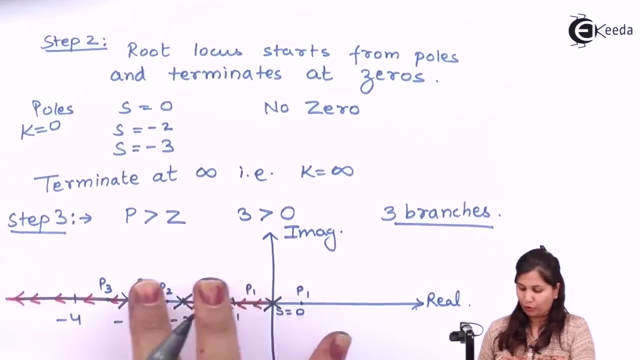 so this is the root locus branches for these three poles. we have known that this is existing between these two parts. okay, so this completes our step number three. now step number four: as you can see in this plot of the roots, that this for these two poles, these two poles are. 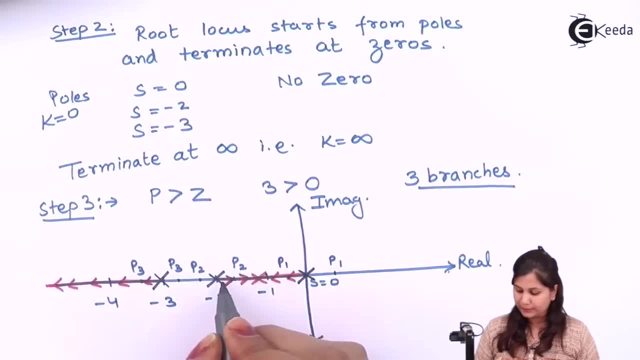 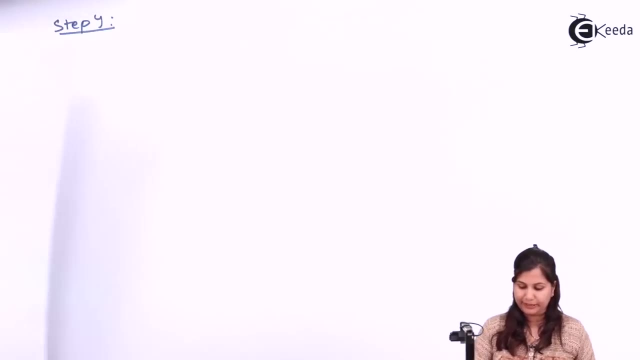 adjacent to each other and these root locus branches, they are coinciding with each other, they are meeting at a point, so so so this point where these two root loci branches are meeting, it is called the breakaway point. so let us calculate this breakaway point. 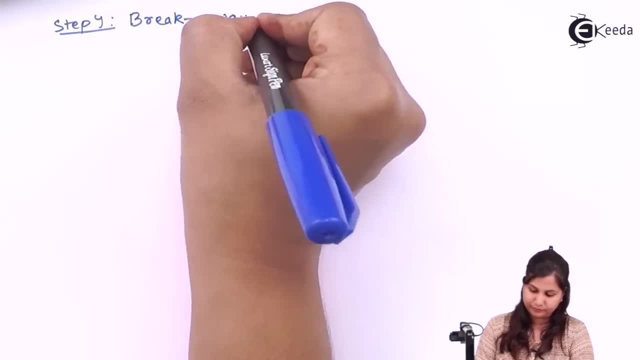 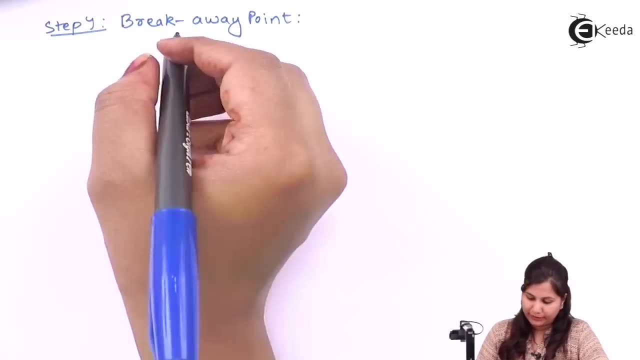 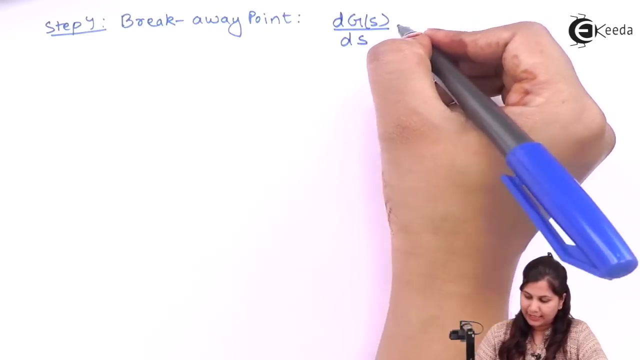 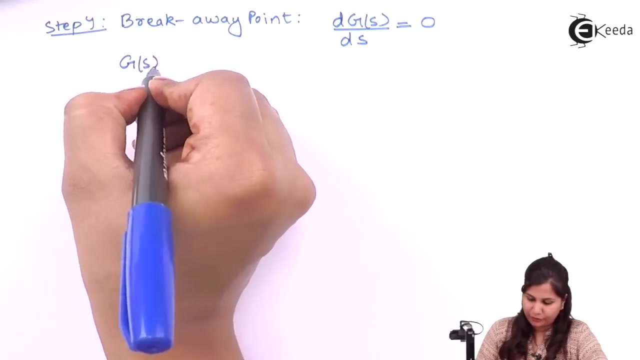 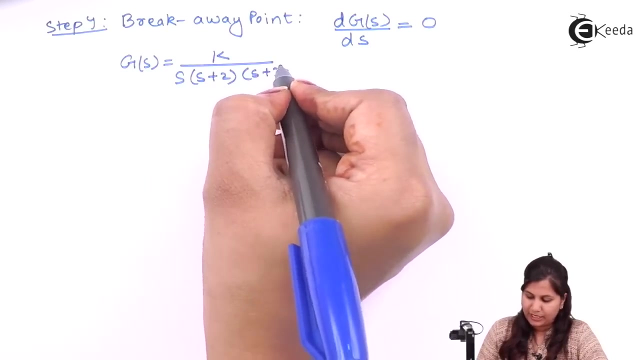 now breakaway point. so the breakaway point is calculated by differentiating the open loop transfer function with respect to s and then equating this differentiation by expectation excited value to zero. so our g s is the Newton's given to us as k upon s s plus 2 s plus three. in the question we are given g s, h s equals to k upon s s plus. 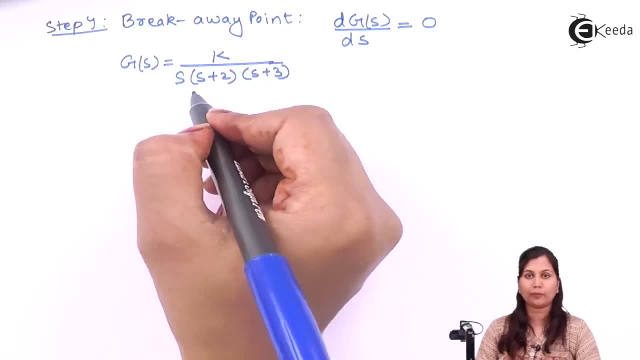 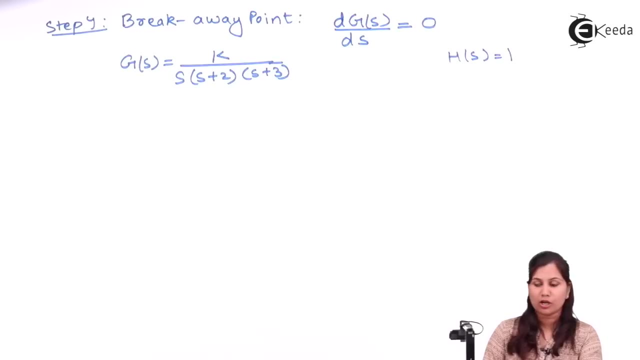 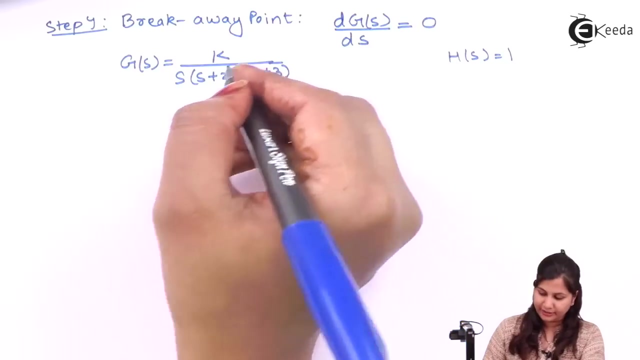 two s plus three. so h s is 1 because it is a unity feedback system. so g s is equal to k upon s s plus 2 s plus three. now differentiate this with respect to unit feedback for the −s X in S orientation, and they are not. variance n gets value of ave x as a function of the. 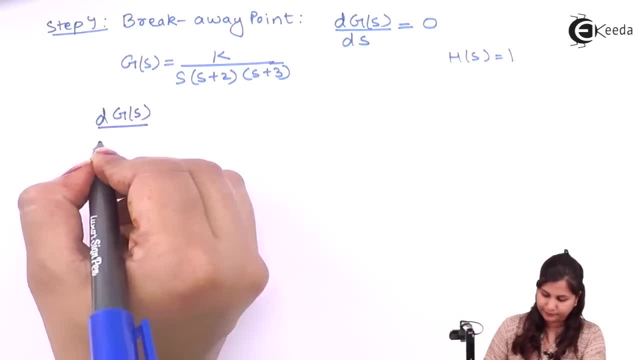 expression. since that given n is a derivative of h S is going to change it. we have to find that. so Chinese H is also an Takes h S you get when the G s need to be this. so specifically to s. There are two methods to find out this differentiation. First is to apply the differentiation. 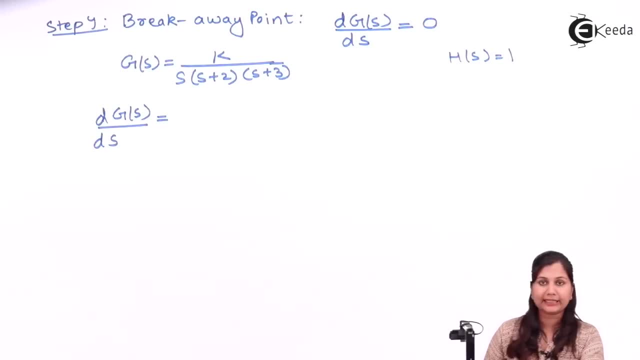 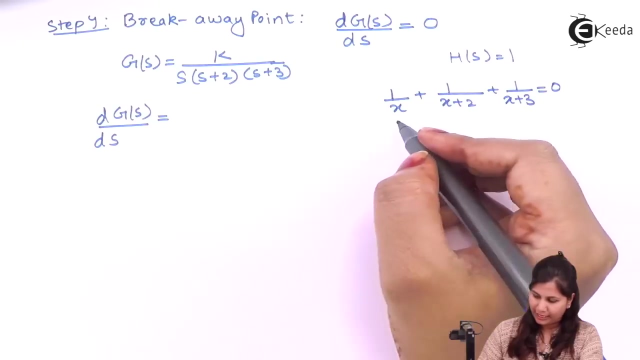 formula and second method is to directly find the breakaway point by letting this s as x 1 upon x, 1 upon x plus 2 and 1 upon x plus 3 equals to 0. So we are having x plus 2, x plus 3. 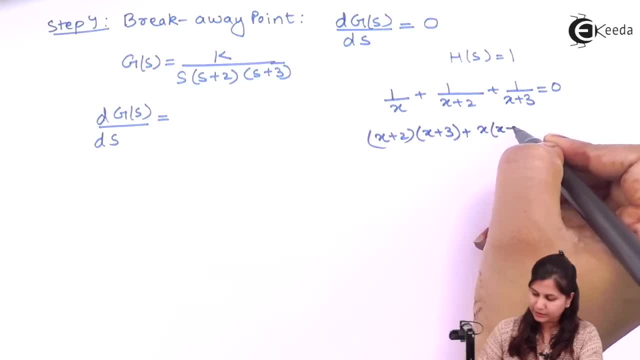 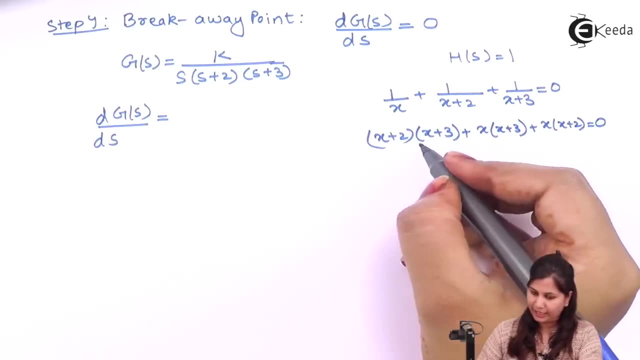 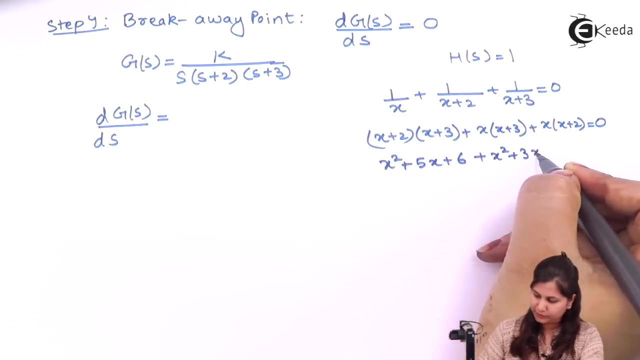 plus x x plus 3 plus x x plus 2 equals to 0.. Solve this: we are having x square plus 5 x plus 6 plus x square, plus 3 x plus x square. So we are having 3 x squared plus 10 x plus 6 equals to 0.. If we solve this equation, we will: 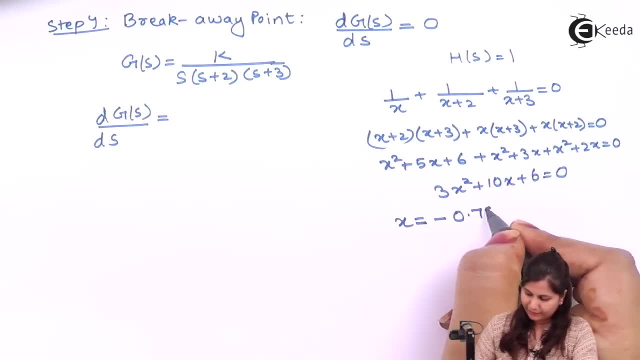 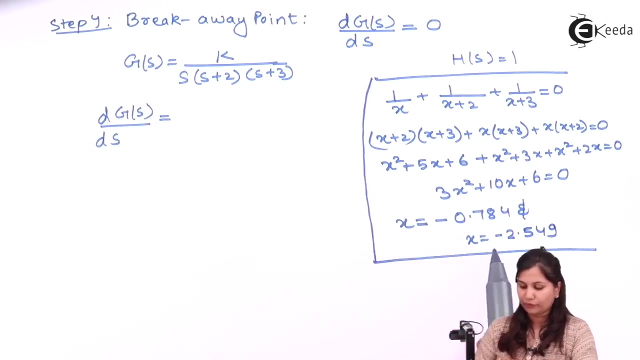 get the value of x as minus 0.784 and x equals to minus 2.549.. So this is one method, or the direct method, to find the value of the x or the value of the x of the breakaway points. Another method is to differentiate it. Apply the differentiation. 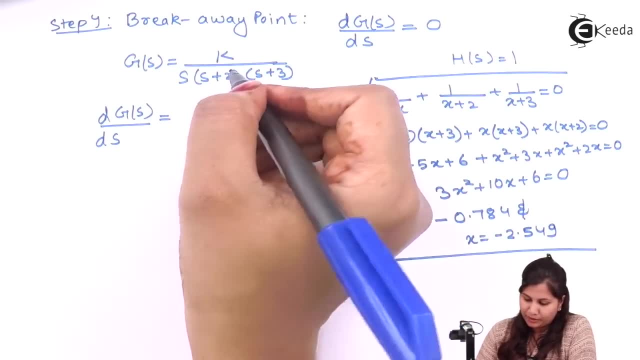 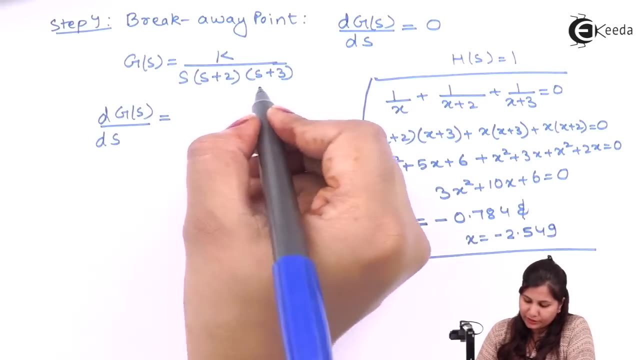 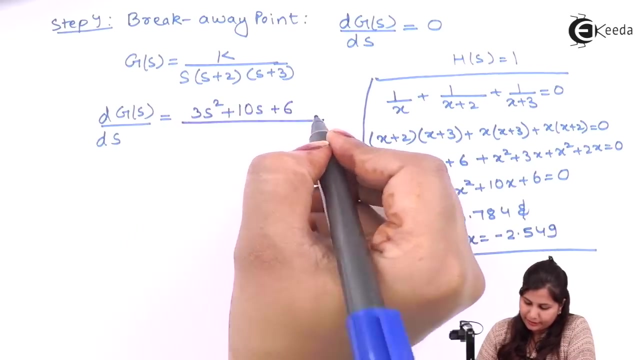 formulas. Differentiation of this will be: k will be 0.. So it will become 0, and the differentiation of this denominator equation is 3s square plus 10s plus 6, divided by s, s plus 2, s plus 3. 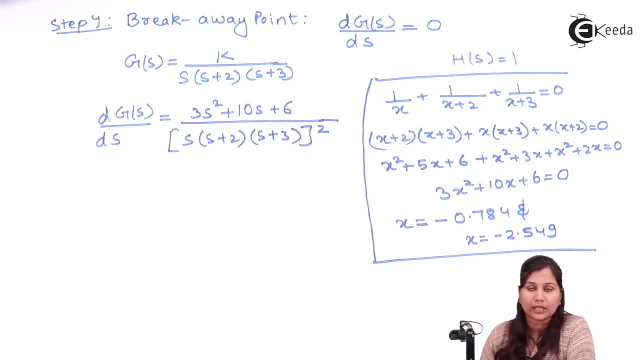 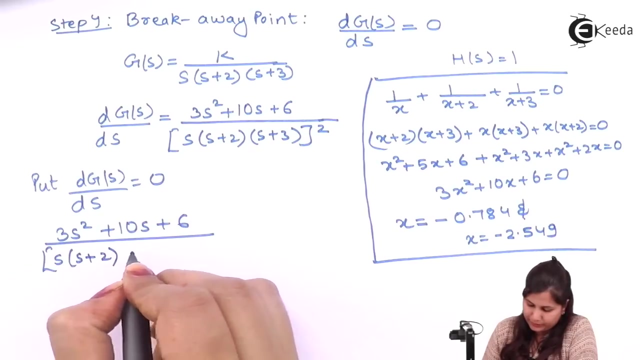 whole square. So this is the differentiation of this open loop transfer function. Now put it to equate it to 0.. So we will get 3s square plus 10s plus 6 upon s s plus 2, s plus 3. 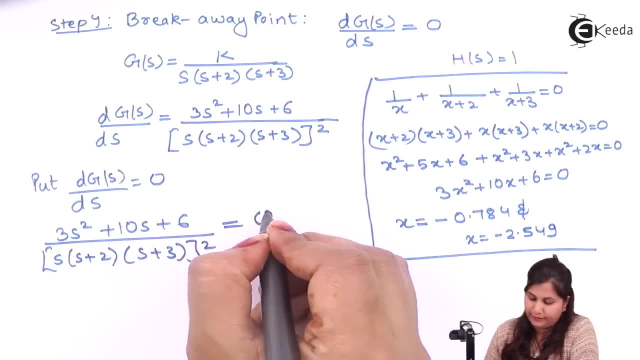 equals to 0. We will be getting 3s square plus 10s plus 6 equals to 0, because when this term goes to the right hand side, it will be multiplied with 0. So it will become 0.. The roots of. 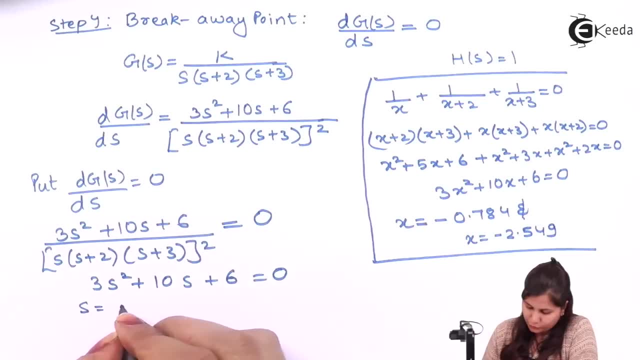 this equation, or the solution of this, will be: s equals to minus 0.784 and s equals to minus 2.549.. So these are the two values of the breakaway points We have. We can use any of the two methods to find out the breakaway points. Either we can apply. 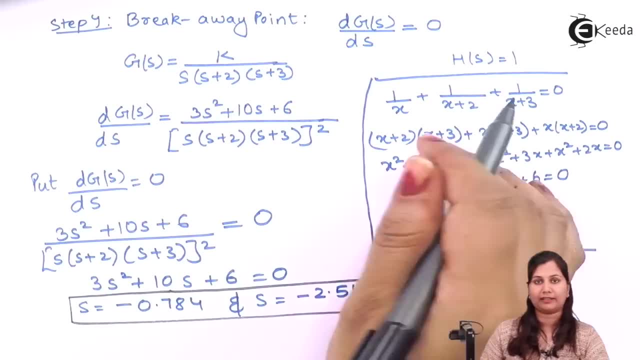 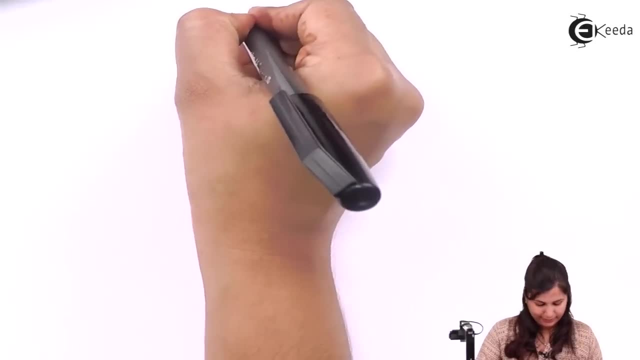 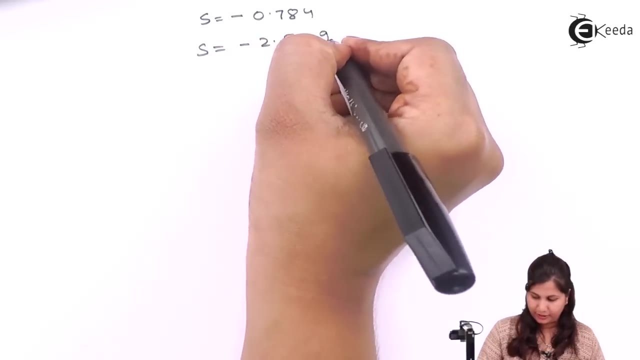 the direct differentiation formulas or we can use this factorization method. Now, out of these two values, that is, s equals to minus 0.784 and s equals to minus 2.549.. Now, if we see our root locus diagram which we have plotted here, 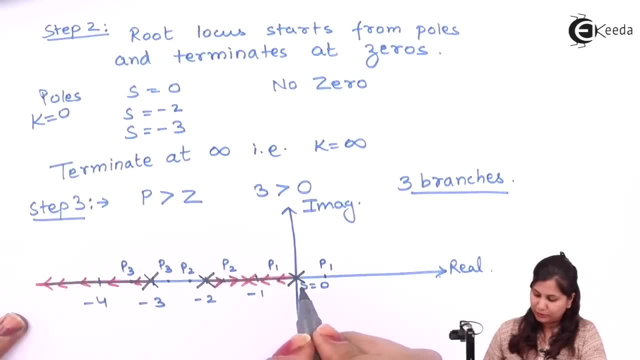 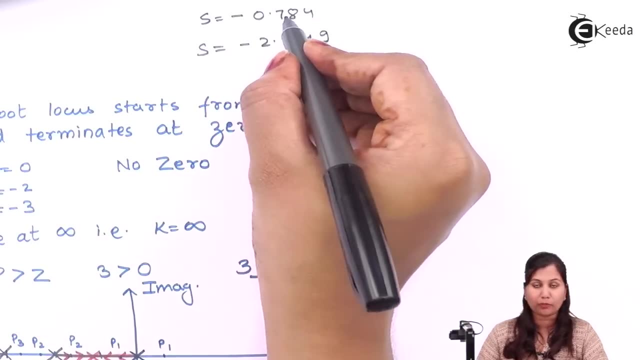 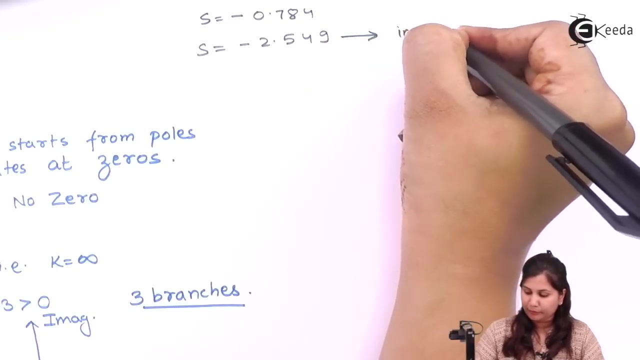 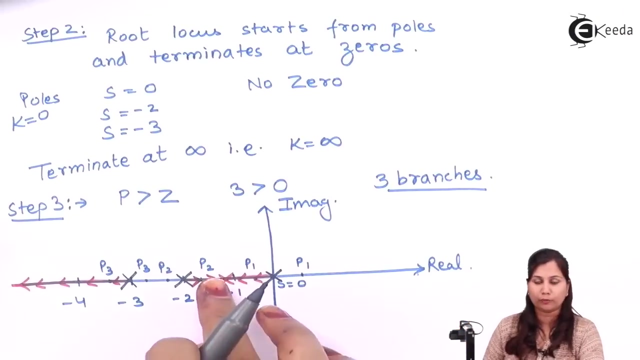 So the breakaway point will be somewhere between s equals to 0 and s equals to minus two, and we are getting the values as s equals close to minus 0.784 and minus 2.549.. So it is not lying between this s equals to 0 and minus 2 point. It is 2.549, which is somewhat. 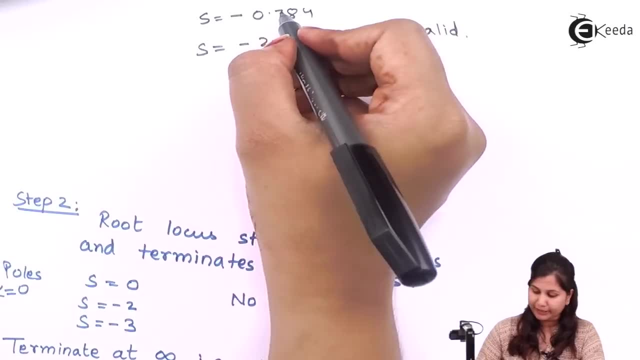 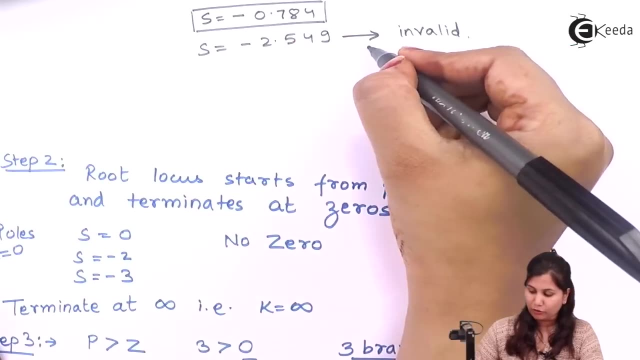 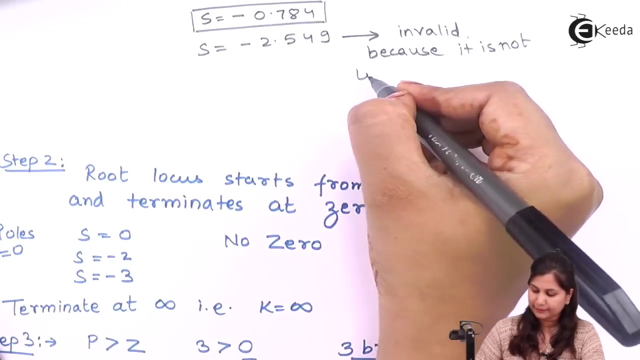 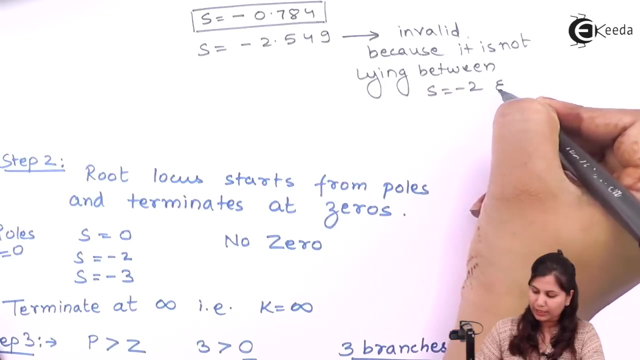 here потому. So our valid breakaway point is: S equals to minus 0.784.. This is invalid because it is not lying between S equals to minus 2 and S equals to 0.. So this is not a breakaway point. 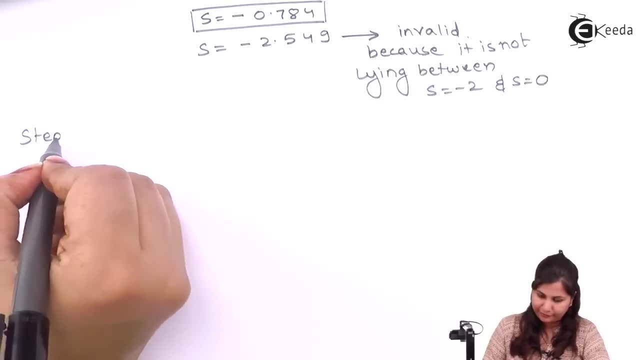 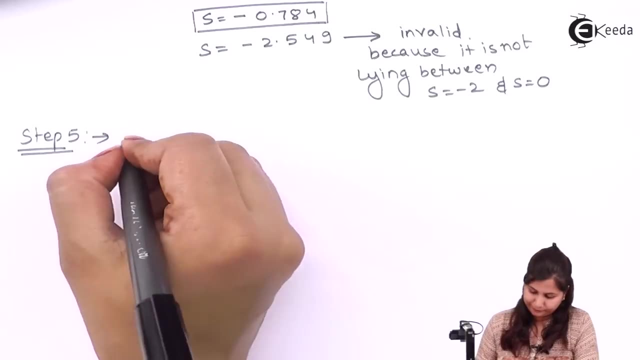 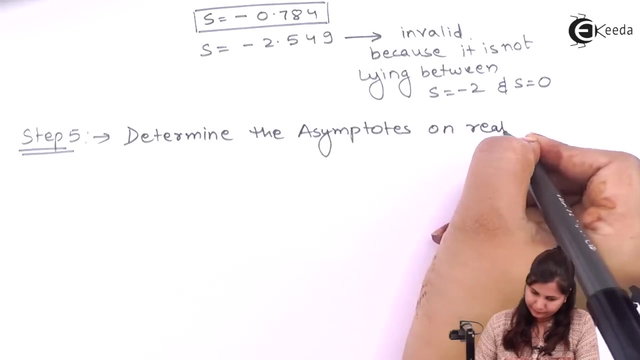 Now our next step is step number 5.. Now we will determine the asymptotes on the real axis. Okay, So for asymptotes we have to first determine the intersection point of the asymptotes with the real axis. So intersection point: 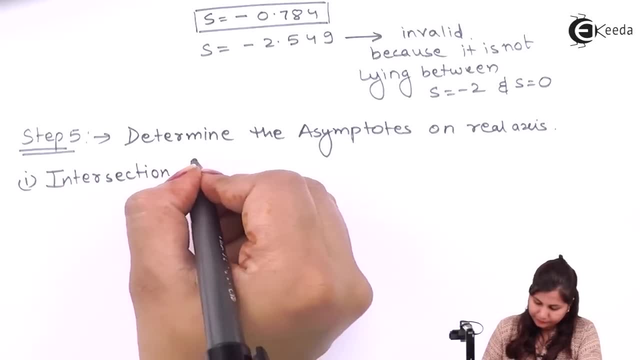 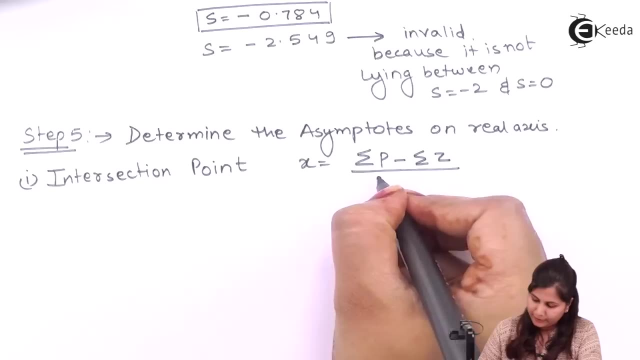 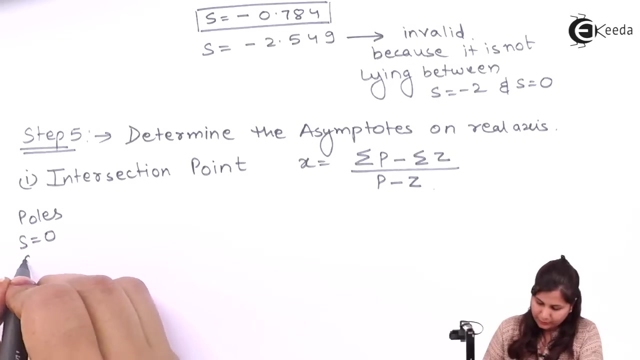 Its formula is: X equals to summation of P minus summation of Z upon P minus Z. Suppose we are having S equals to 0, S equals to minus 2 and S equals to minus 3.. So summation of P will be 0, minus 2, minus 3, that is, minus 5.. 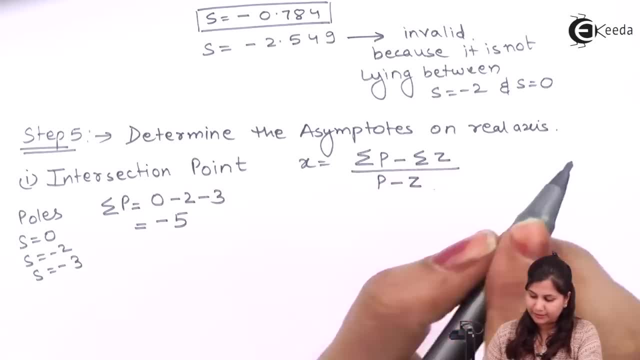 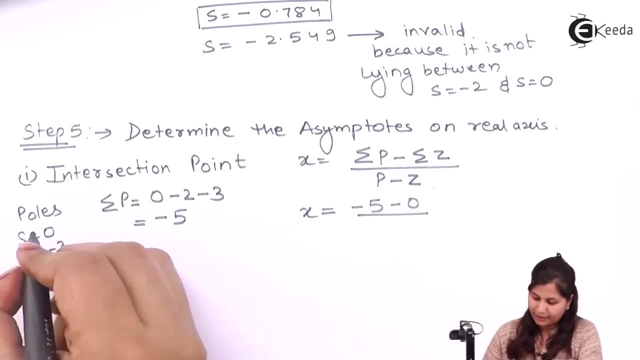 And 0.. 0.. 0. 0.. because we are not having any 0, so it will be. its summation will be 0, so it is minus 5 minus 0. number of poles are 3, so p equals to 3, and number of zeros is 0, so it is 0. so we are getting here. 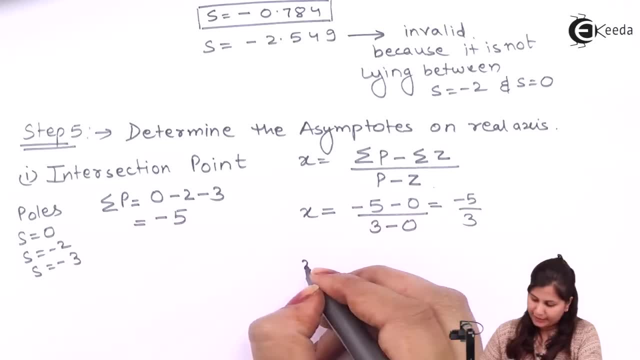 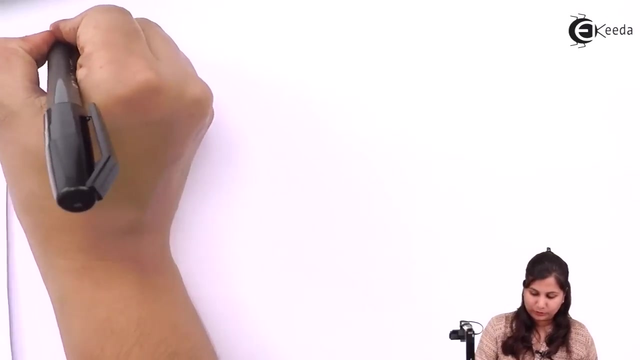 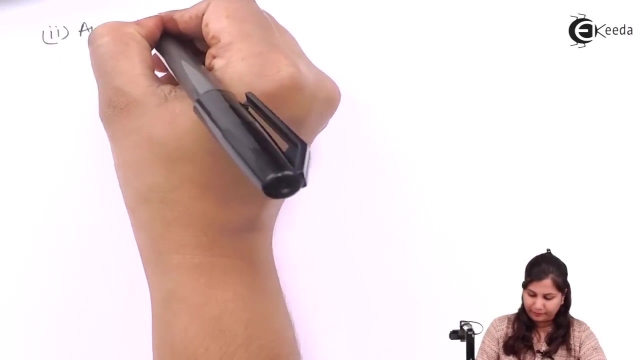 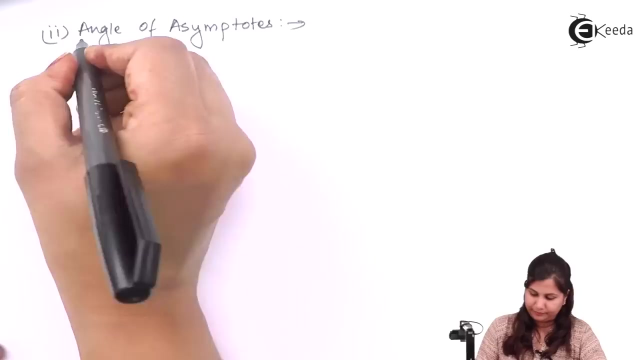 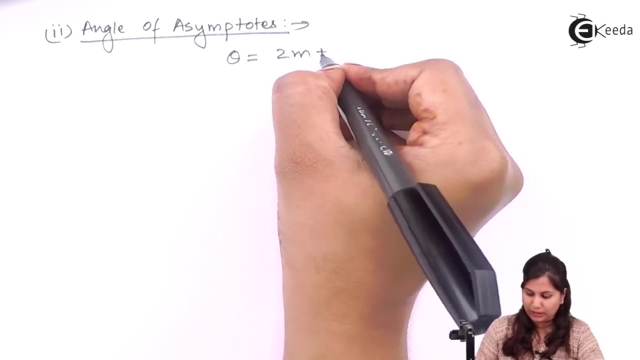 the value as minus 5 by 3 or x, is equals to minus 1.667. so it is the intersection point of the asymptotes with the real x's. now, in second part, we will find out the angle of the asymptotes. how we can find out the angle, we have a formula for it. theta equals to 2m plus 1 into 180 degree. 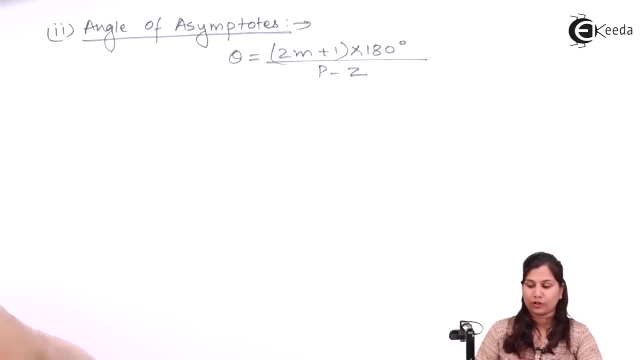 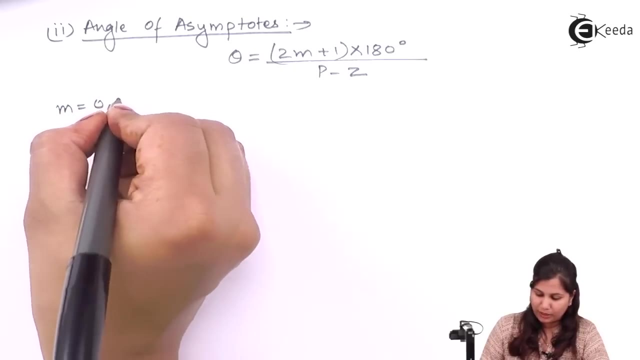 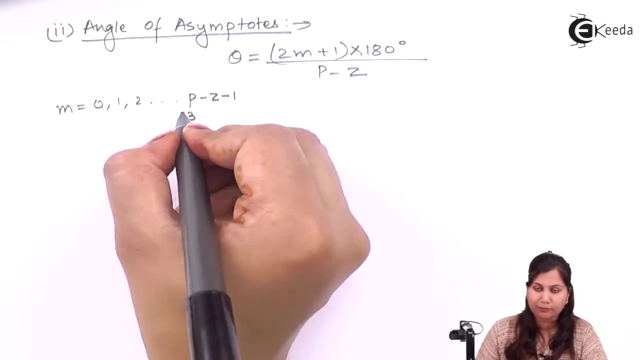 and divided by p minus z. so it is the formula for the angle of asymptotes. here m will be equals to 0, 1, 2 till. we are having p minus z minus 1, so p- we are having 3 poles and zeros- is 0. 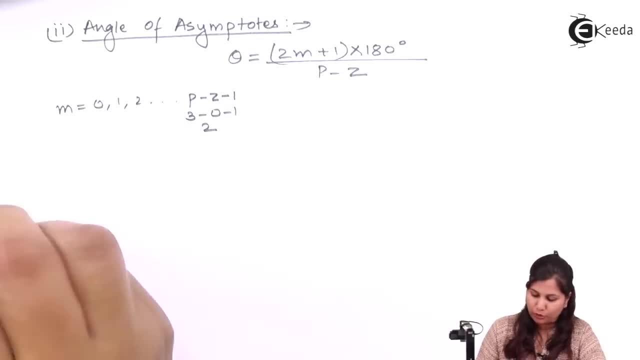 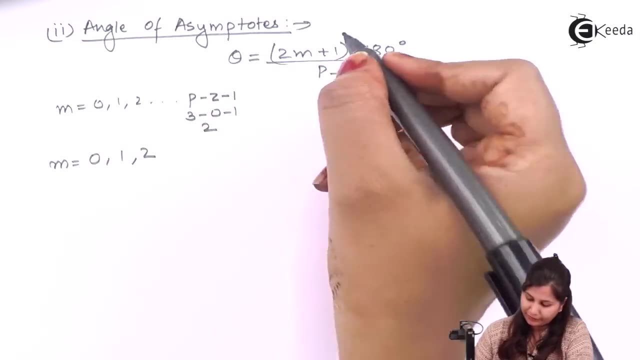 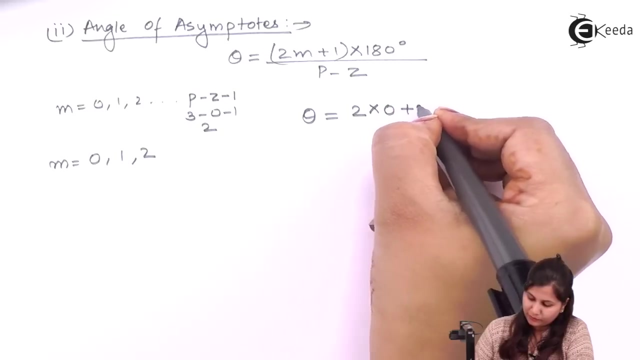 and then minus 1, so 3 minus 1, 2. so the value of m will be 0, 1 and 2. okay, the value of m here, theta, is equals to 2. first putting m equals to 0. so 2 into 0 plus 1 into 180. 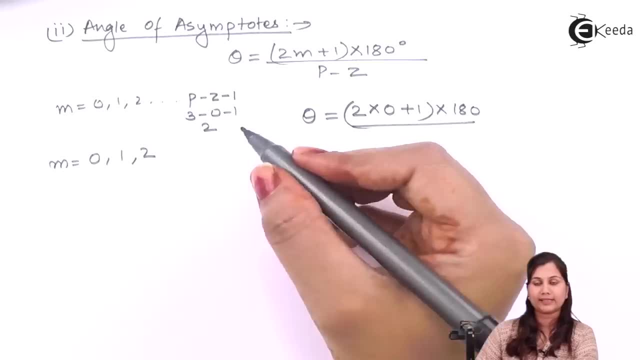 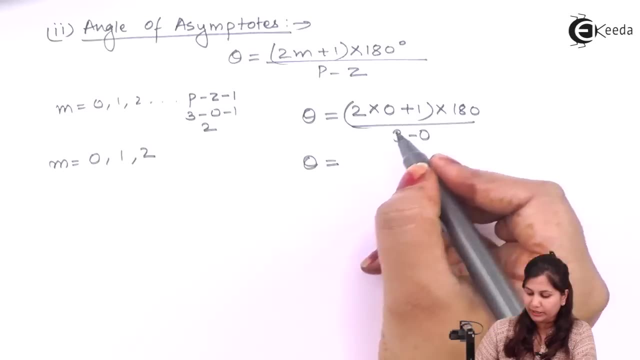 upon p minus z. number of poles is 3 and number of zeros is 0, so theta will be 0 plus 1 into 180, 180 by 3, so it will be 60 degrees. for m equals to 0, for m equals to 1. 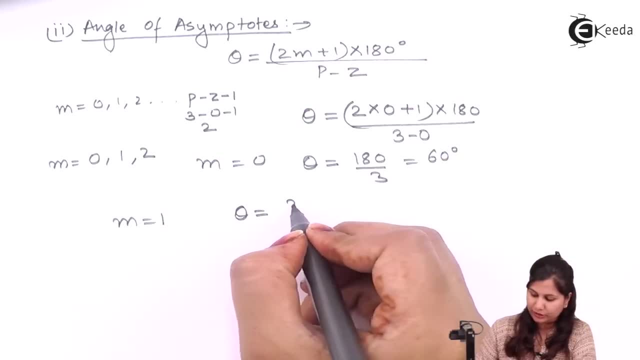 2 into 1 plus 1, that is 3 into 180 upon 3. so theta will be 180 degrees for m equals to 2. put here 2, 2, 0, 4, 4 plus 1, 5, 5 into 180 by 3. okay, so here we are getting the. 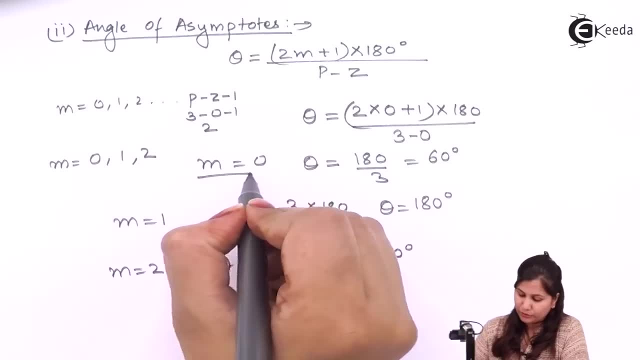 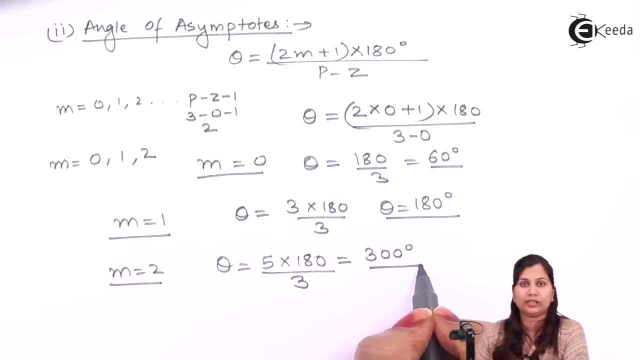 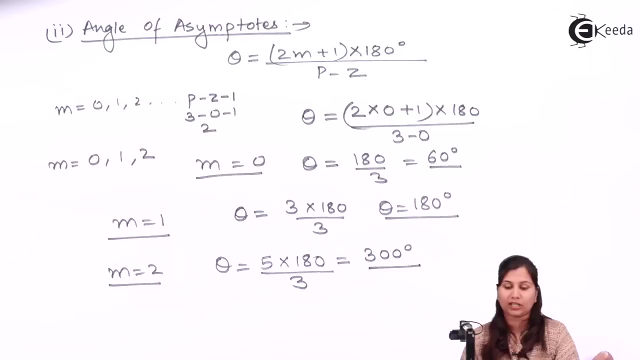 value as 300. so for m equals to 0, theta is 60 degree. for m equals to 0, theta is 60 degree. for 1, theta is 180 degree. for m equals to beta is 300 degrees. so we have obtained 3 loops of the asymptotes for the 3 branches which we are getting in the root. 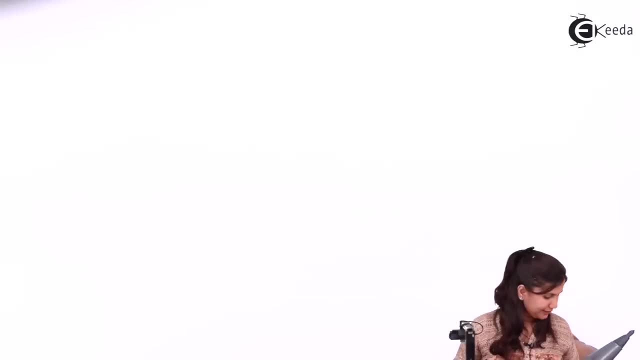 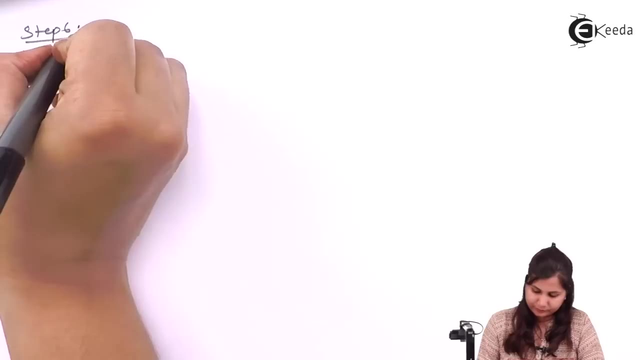 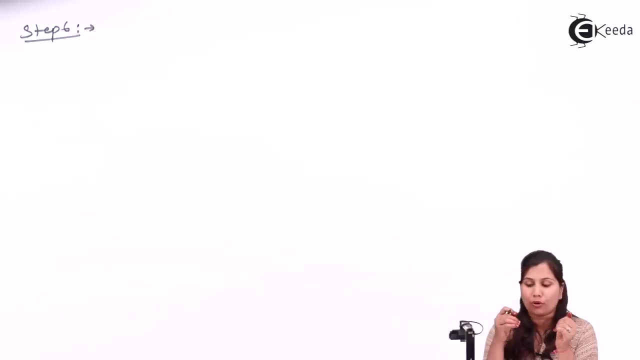 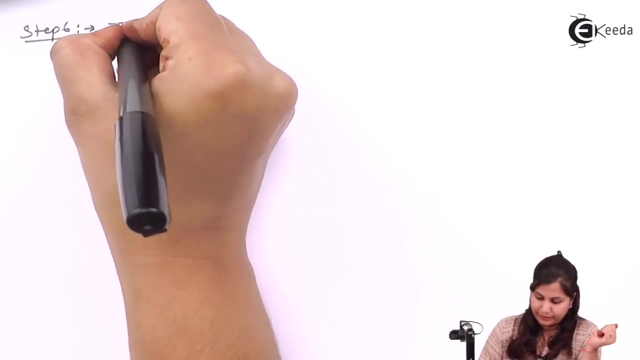 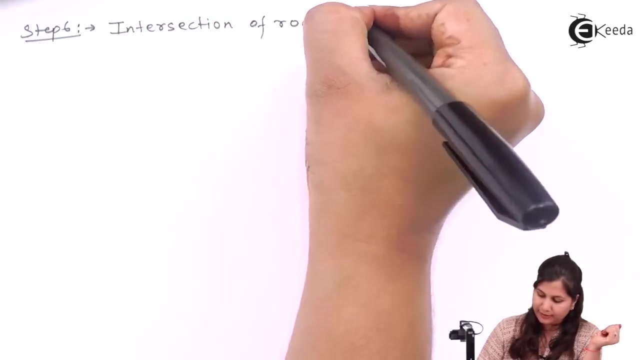 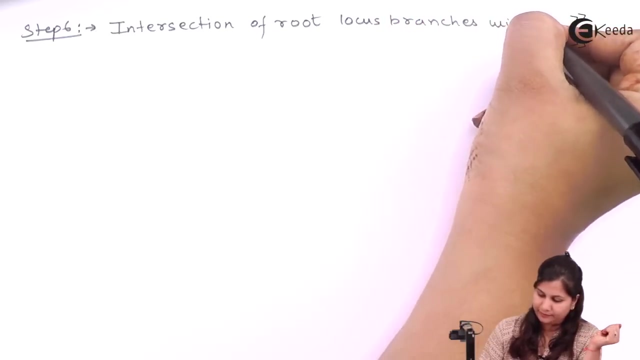 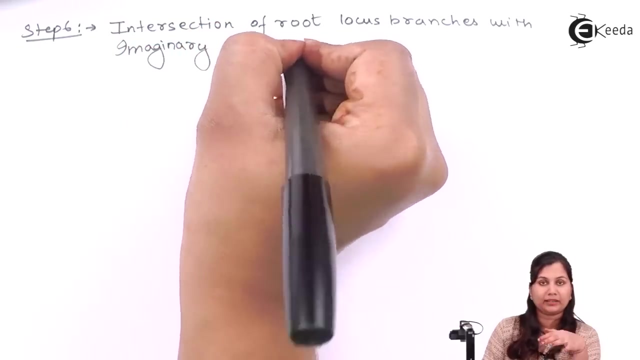 locals. now our next step is, that is, step number 6. now, in step number 6, we will determine the intersection: intersection of the asymptotes, or the branches of the root locus with the imaginary axis. Intersection of root locus branches with imaginary axis. We were having two methods to find out. 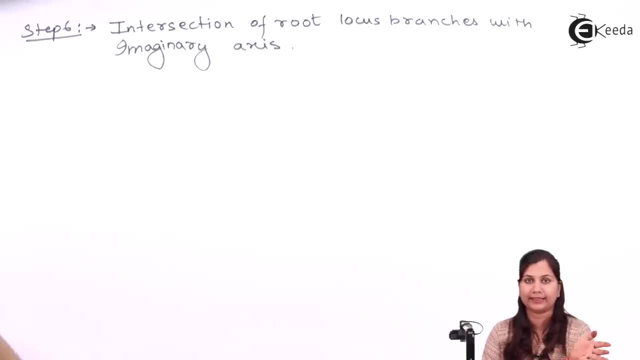 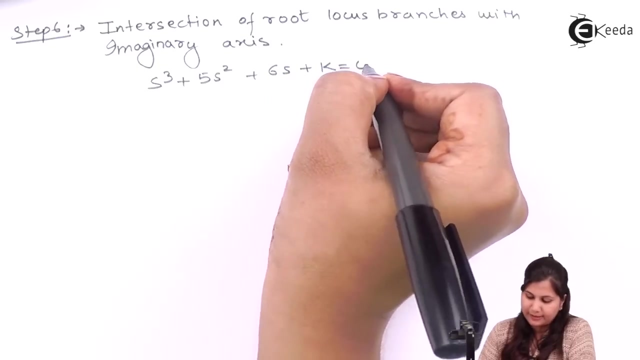 this: First was to put s equals to j, omega in the characteristic equation and second was to use the root stability criteria. So here we will use the root stability criteria to find the intersection point. The characteristic equation of this system was sq plus 5s. square plus 6s plus k equals to 0.. 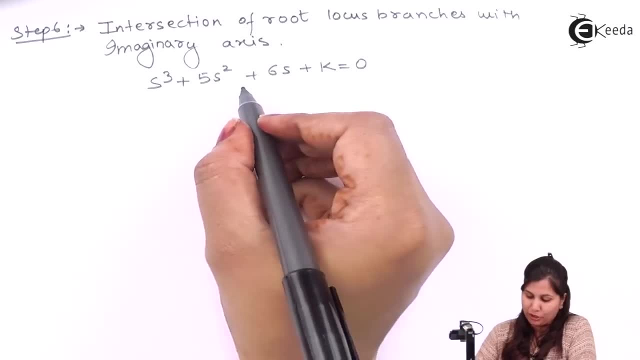 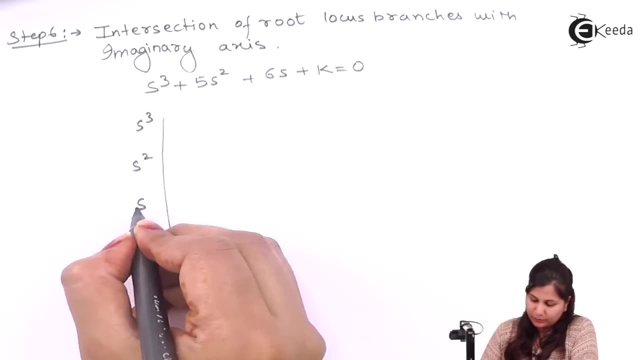 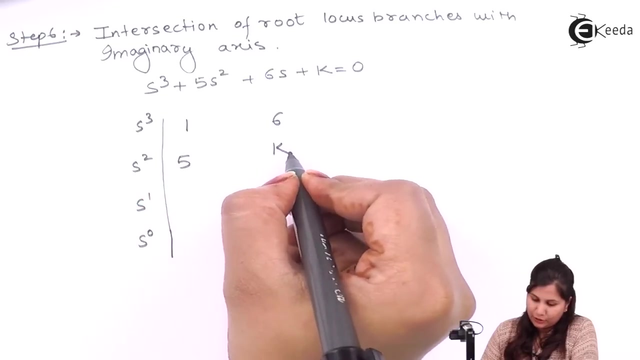 Characteristic equation we have already obtained in the first step, So use this characteristic equation. form the root array s cube s square s1, s0.. Coefficient of s cube is 1, then 6, here 5 and k, so it will be 30 minus 5, 6 or 30 minus k. 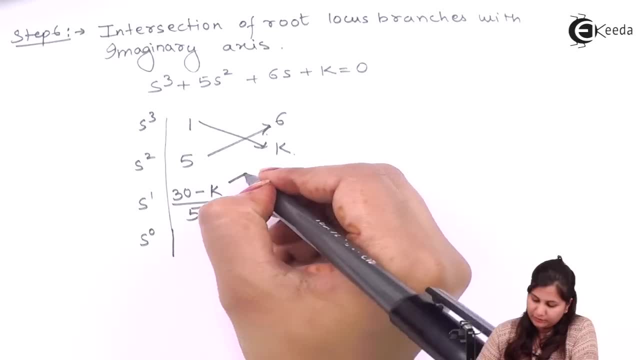 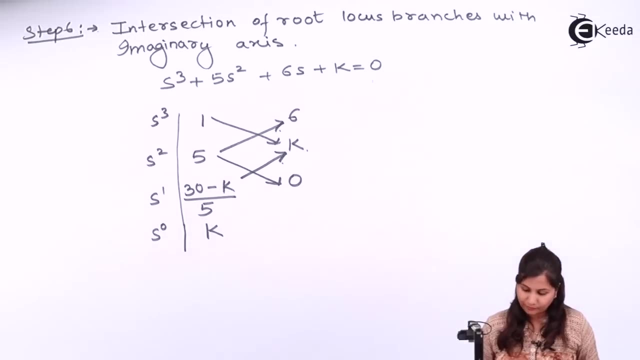 upon 5, it will be 0. then 30 minus k into this and 5 into 0 is 0. so here we will get k. So this is the root stability criteria. we have formed the root array. Now for the system to be. 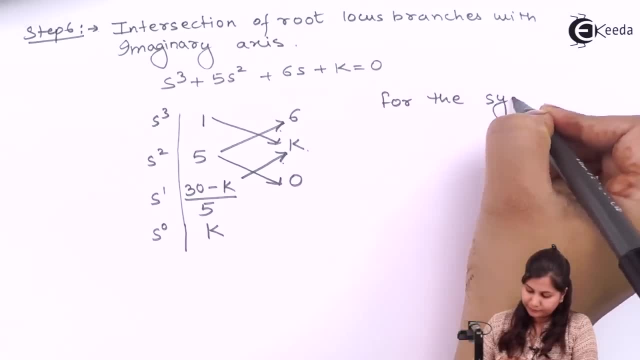 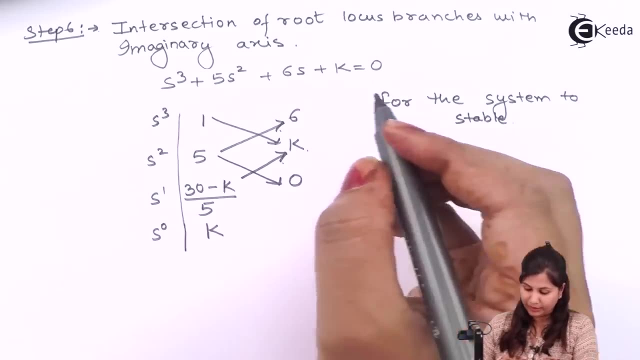 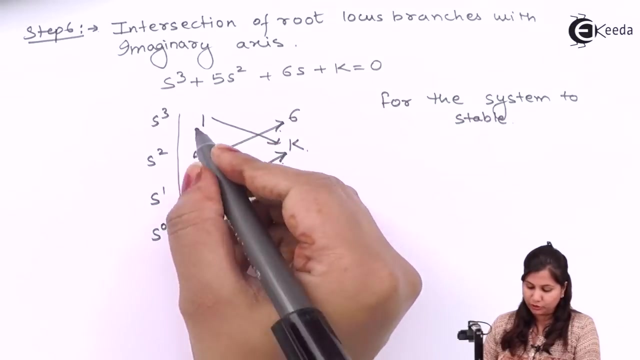 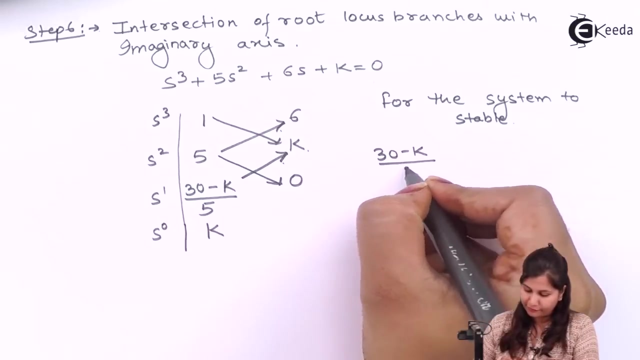 stable. so in a root stability criteria the system is stable. when the in the first column there is no sign change, that is here we are having positive. so all the coefficients, they should be positive. That is greater than 0. so 30 minus k upon 5 should be greater than 0 and k should be greater than 0. 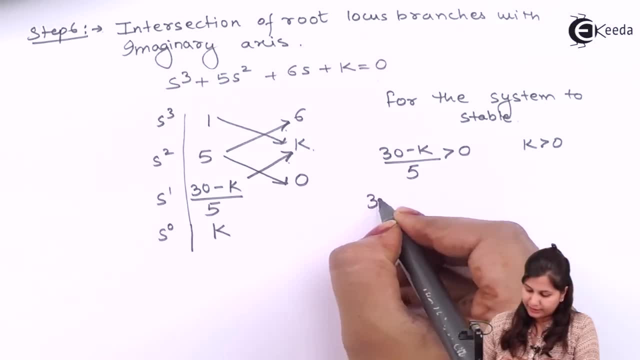 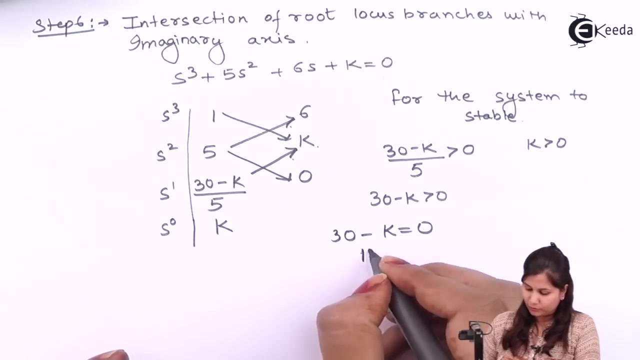 okay, so from here we are getting the value as 30 minus k, greater than 0, so k should be equals to greater than 0. or it should be equals to 0, so 30 minus k, it should be 0, that is, k equals to. 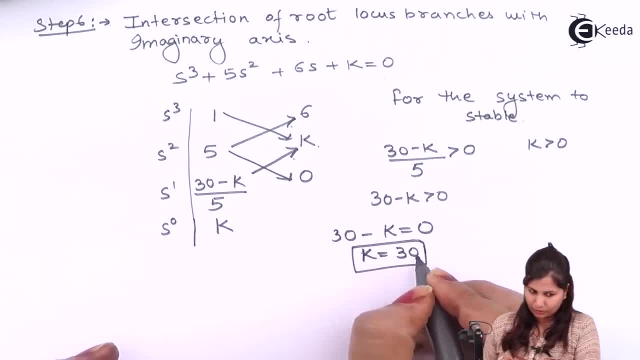 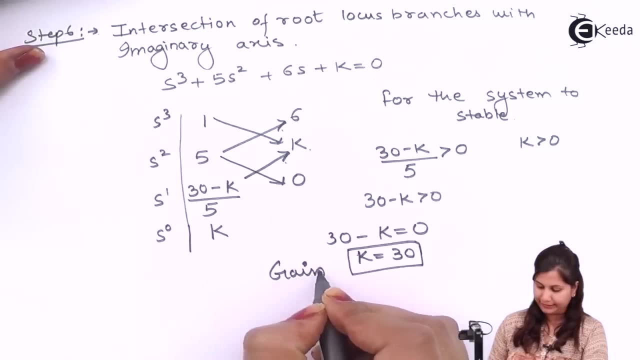 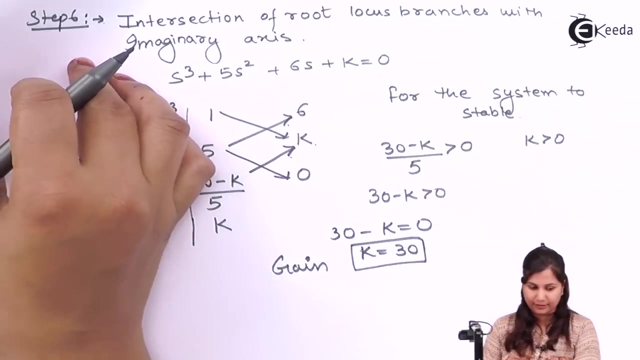 30. 30., 30., 30.. okay, so we have obtained the value of k. that is our gain. and this is the intersection of the root locus branches with the imaginary x's. now, for this, k equals to 30. we are going to determine. 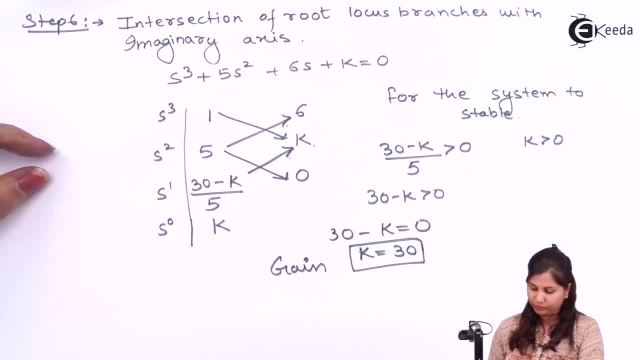 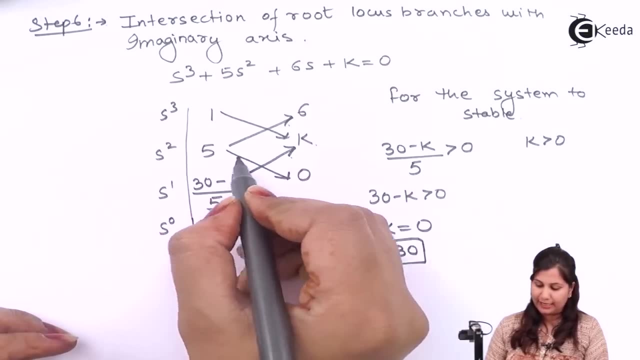 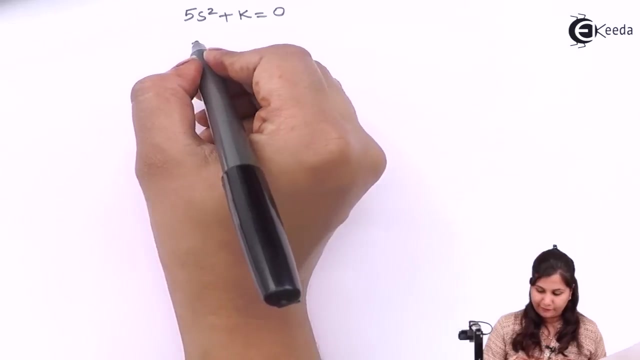 the value of the omega s value. okay gain we have obtained. write the subsidiary equation, use the row just above this and equate it to 0. so 5s square plus k equals to 0. so it will be 5s square plus 30 equals to 0. 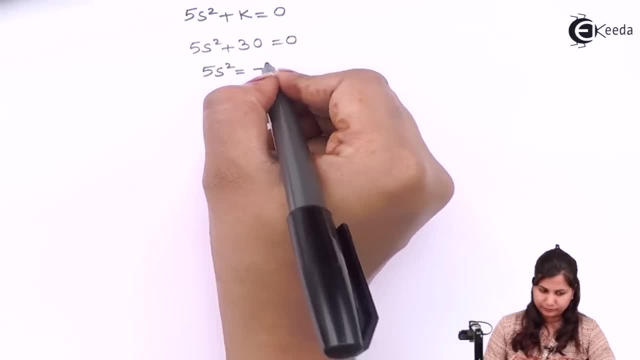 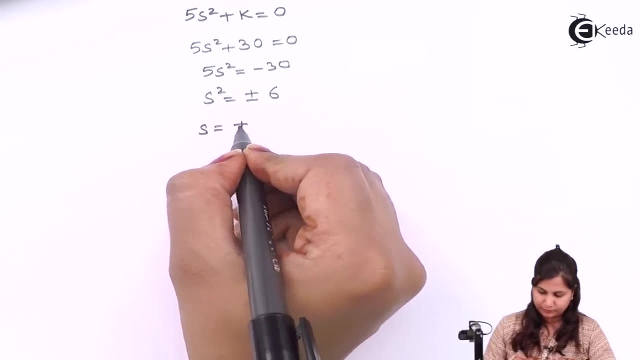 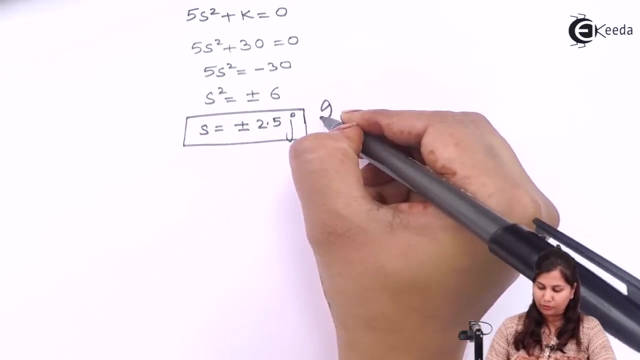 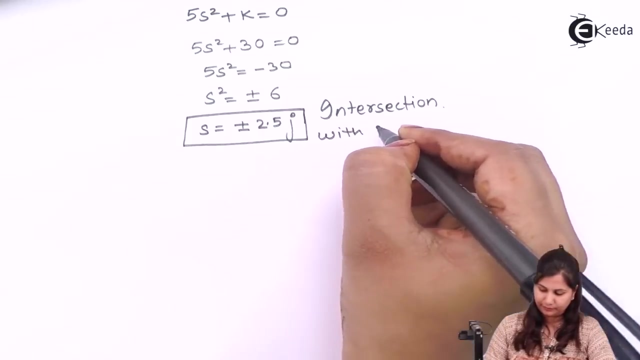 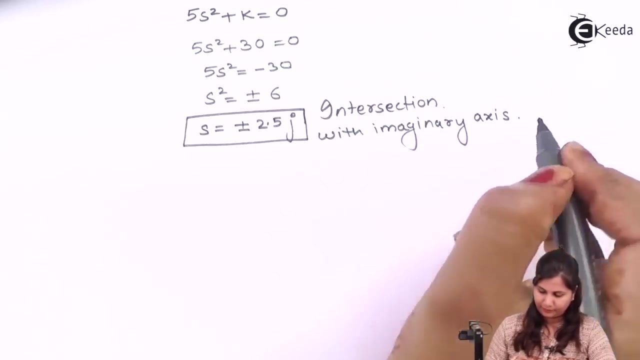 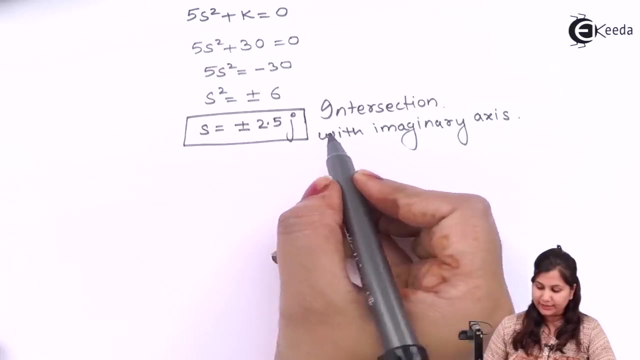 so this is the intersection point, or intersection with the imaginary x's. so s is what sigma plus j's omega, and here, because it is intersection with the imaginary axis, so s is equal to sigma plus j omega. here it is. 4th point: sin. Sin is equal to zero. so its will be catch of point of intersection with the imaginary axis. so s is 2 power s. add up to k riding with pi n and add up to k riding with pi n and add above just 5s square, that equals to 655不好意思, we only have notice that the vector cos qué in空 name is also constant, which decides whether sigma is equal to sigma or j is going to counter square. be forever Here. de duras is equal to I Juzi, because the intersection is in the imaginary angle Number one: plating of the vertex, making of, In other words, this sign: dias Justice's. 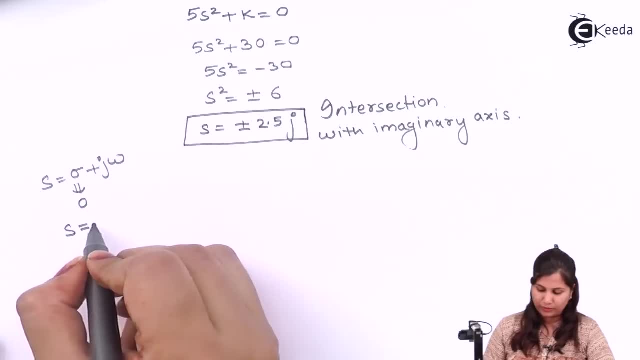 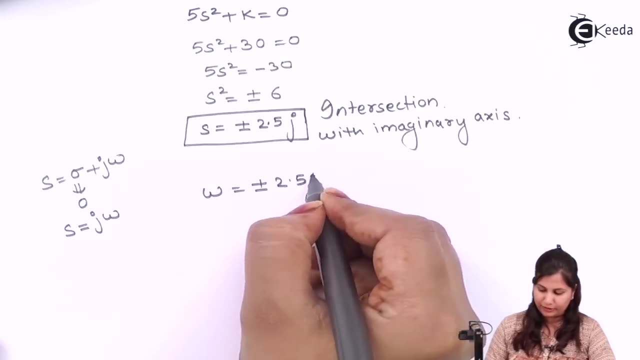 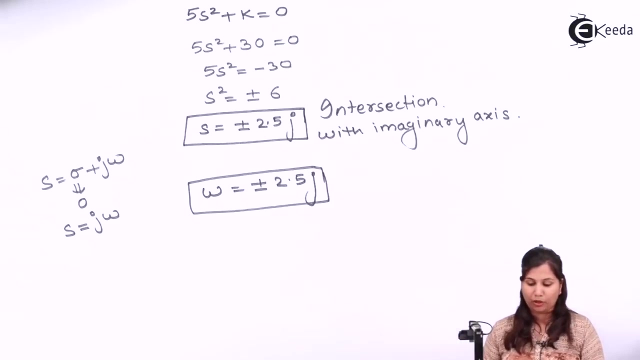 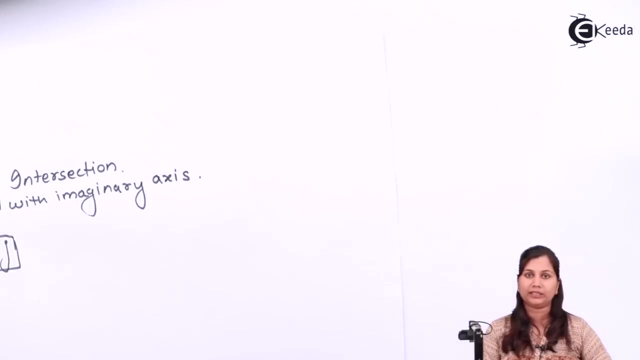 imaginary axis. so s is equals to here j, omega. so omega will be equals to plus minus 2.5 j. so we have done all the steps for this root locus. now let's plot this root locus diagram. we have obtained the breakaway point, we have obtained the intersection, we have obtained the. 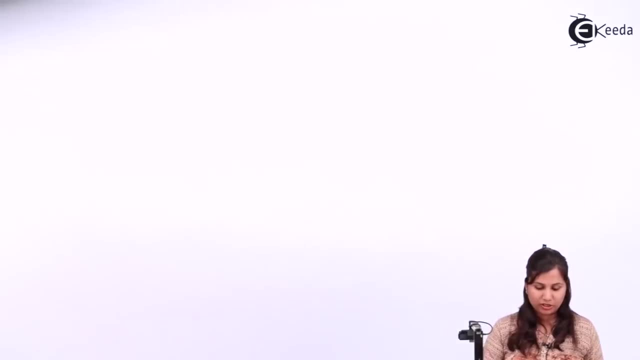 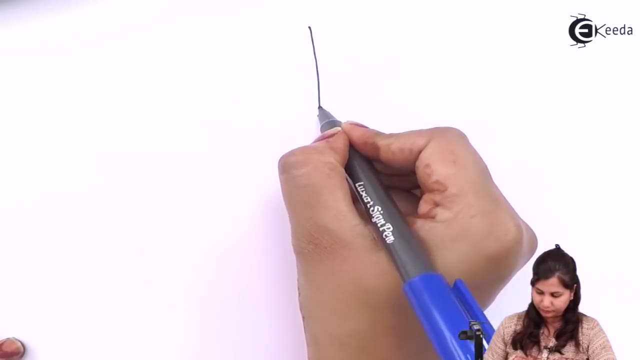 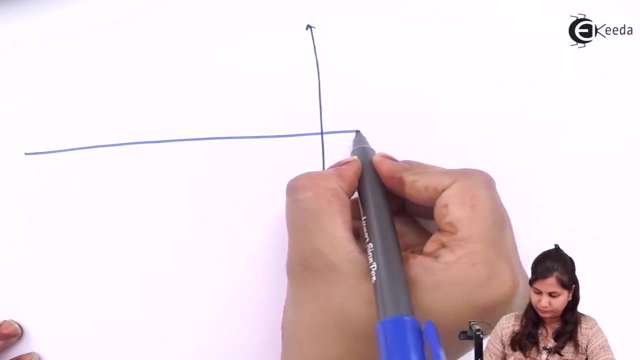 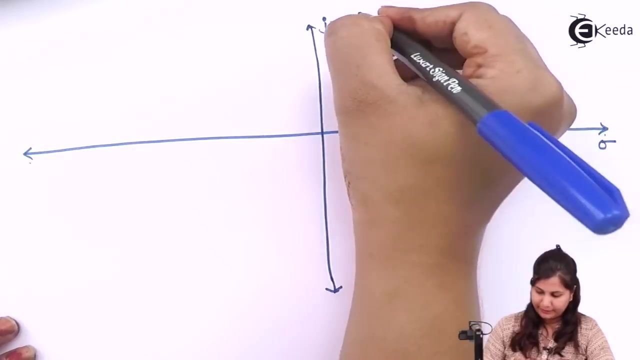 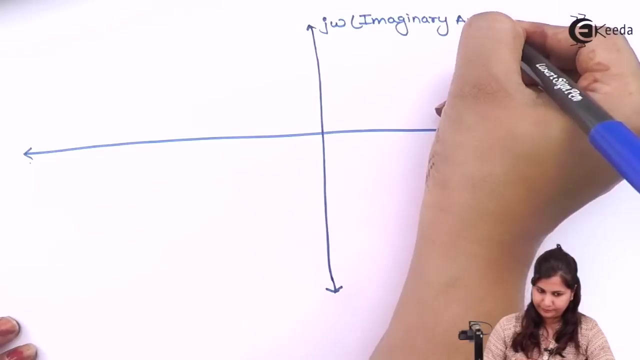 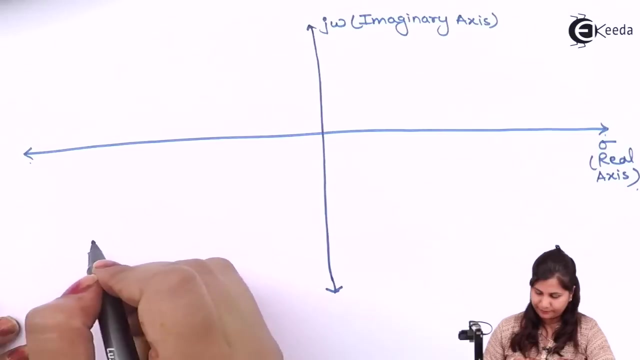 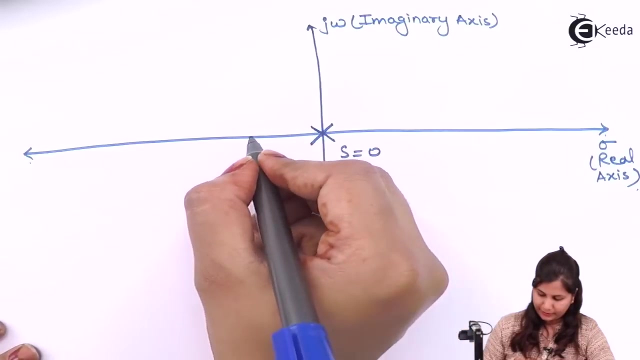 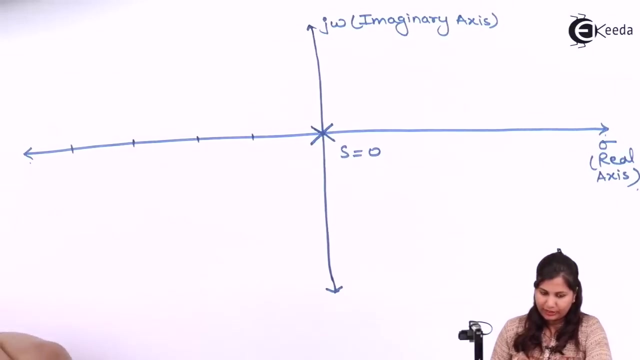 asymptotes, all the steps we have followed. now just sketch this root locus. this is j, omega and this is sigma imaginary axis and this is real axis. okay, s equals to 0. we are having a pole, then minus 1, minus 2, minus 3, minus 4, and this is infinity. so we were having s equals to minus 2. 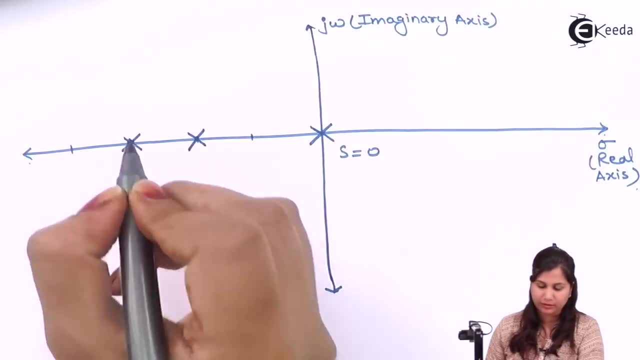 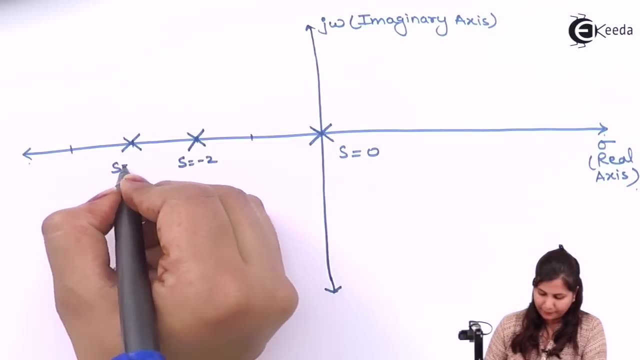 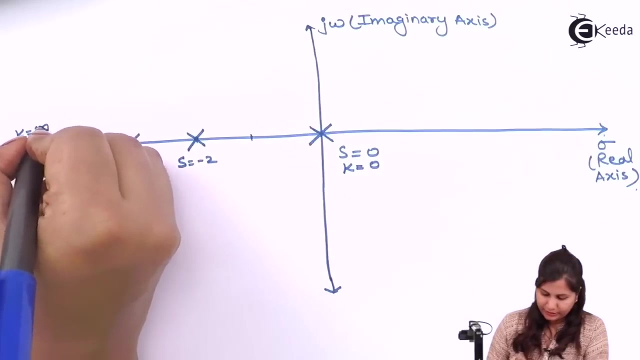 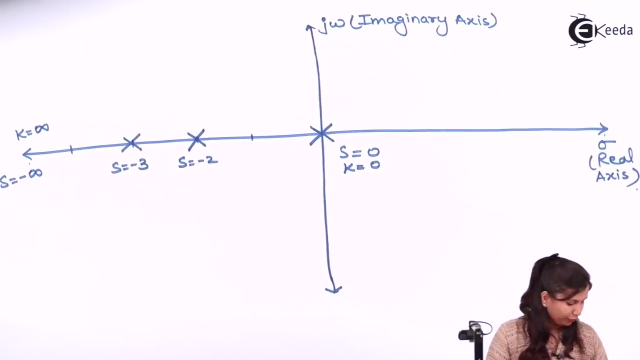 and we are having s equals to minus 3.. as a pole, okay, s equals to minus 2, s equals to minus 3. this is for k equals to 0 and for k equals to infinity. we are having s equals to minus infinity. direction of the root locus we have obtained in our first step. 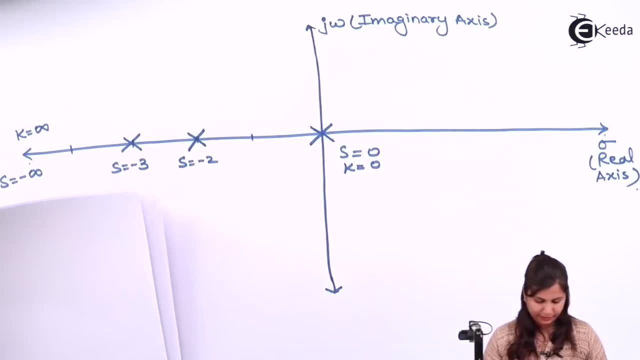 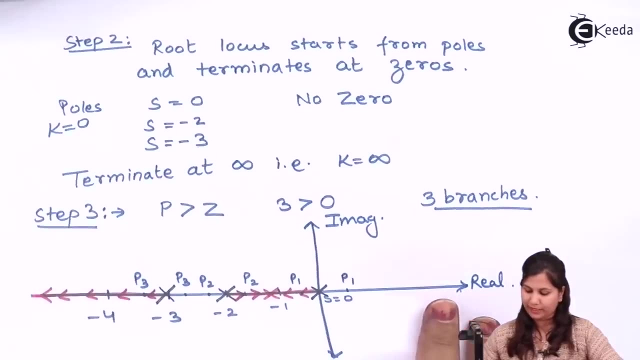 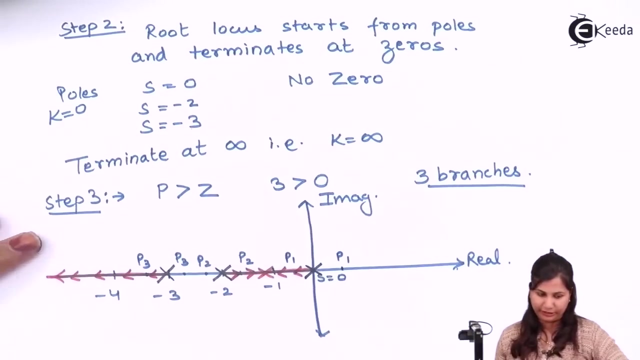 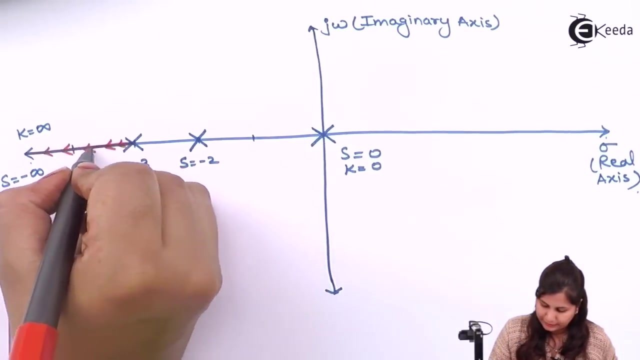 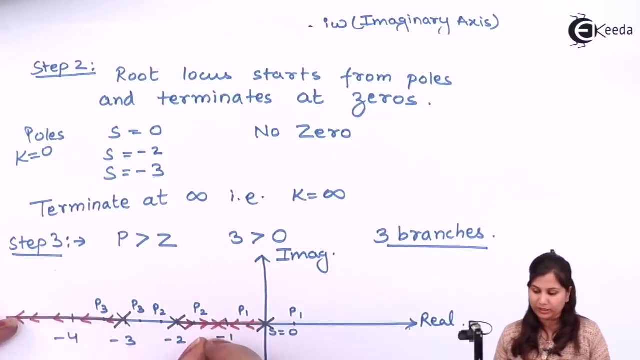 here we have obtained that, the direction, direction of the root locus. we have obtained already in our step number 3- that for s equals to minus 3, it will be towards infinity. so we will plot here again this: okay, so it will be like this: for s equals to minus 2 and s equals to 0, it will be towards each other. so it will be like: 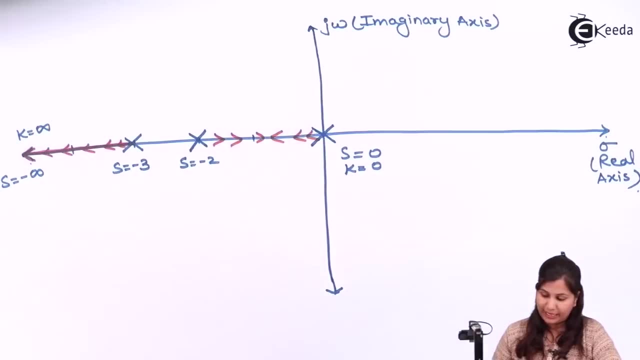 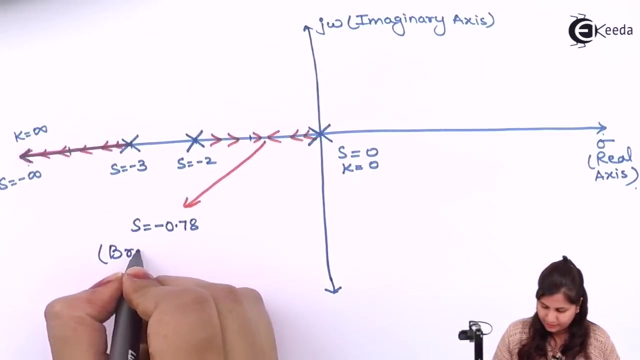 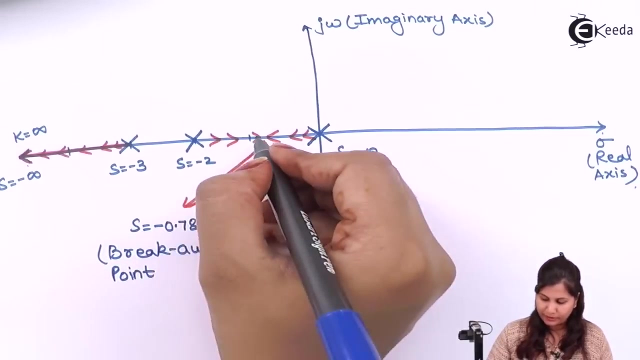 towards each other. and here we are having the breakaway point where the two root locus, for due to these two poles, they are breaking. so this breakaway point is what s equals to minus 0.78? this is our breakaway point. so from this point, that is minus 0.78. these two, both locus 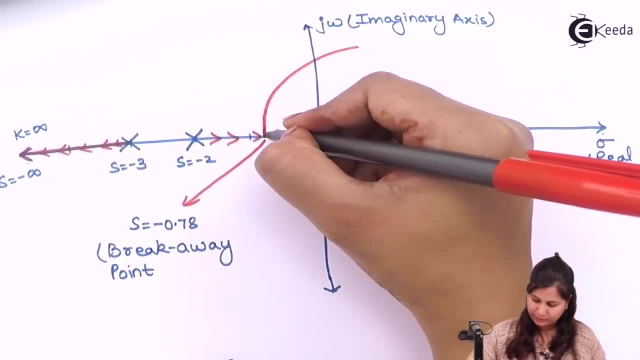 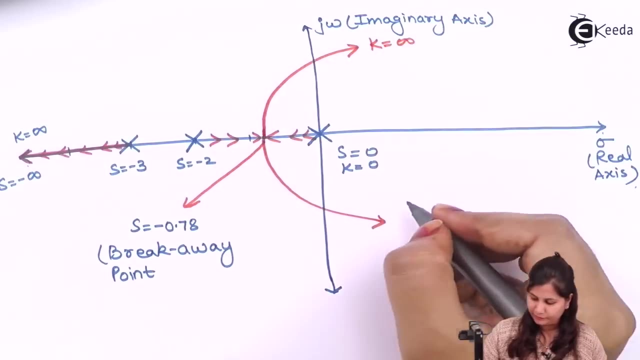 they will be diverging and they are terminating at k, equals to infinity. now these two branches equal the g axis. they are also Bes edible and the two branches are perfect in this situation, especially for both locus weight, such that these two branches are completelyspeaking near each other. 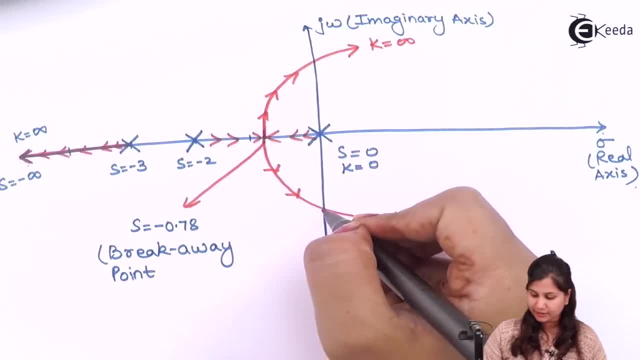 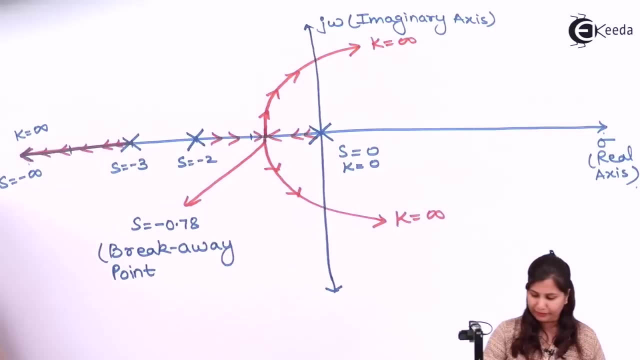 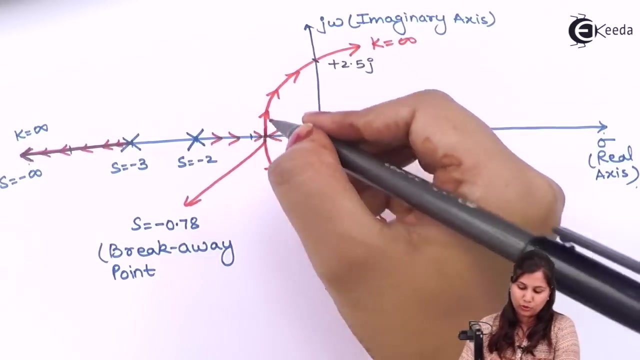 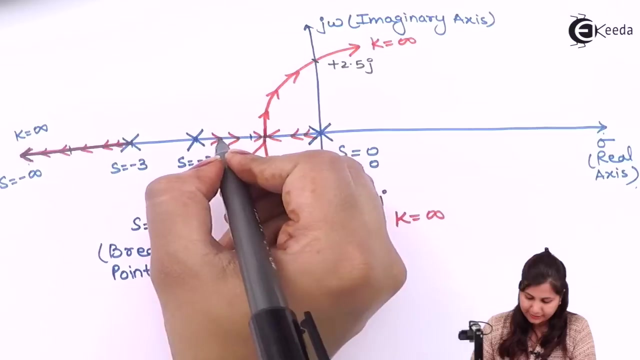 So branches will intersect the imaginary axis on the points which we have calculated as plus, minus 2.5 j. So this point is plus 2.5 j and this is minus 2.5 j. Okay, Now, on these two, two glocus branches, we are having the asymptotes, Okay, And these asymptotes will intersect the 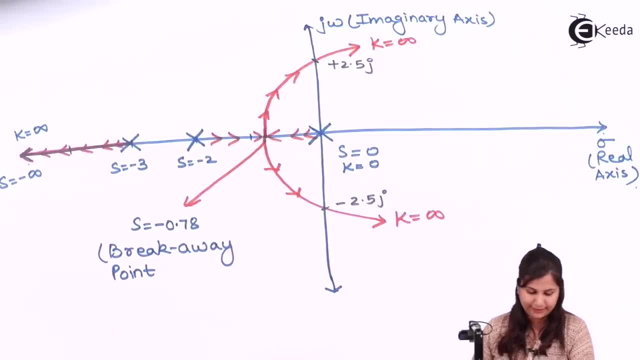 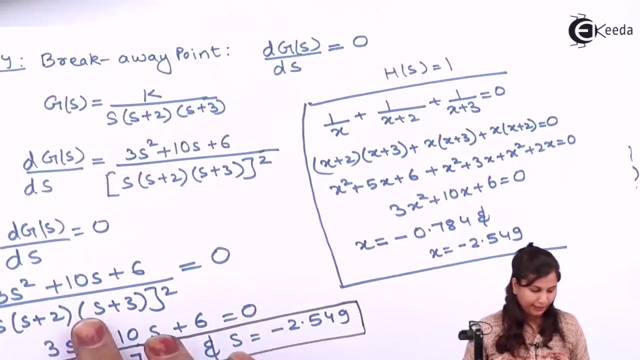 real axis at a point minus 1.67 which we have obtained in our step number. Here we have obtained that breakaway point we have already obtained here, as this minus 0.784 and angle of asymptotes which we have obtained is equal to minus Пa, that is the bread default angle of Asymptotes. 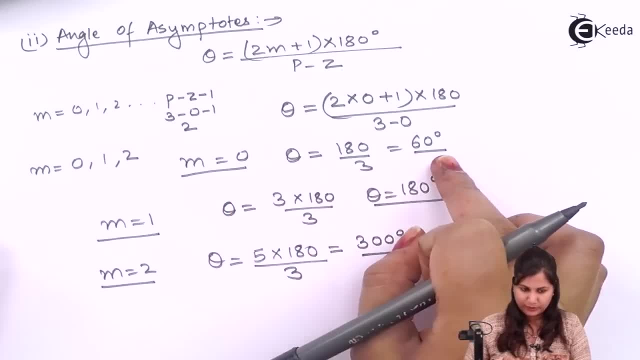 I have used the Asymptotes model in this case. Oops, there we go. So we have интересatt larsc to find this worked out here. So over here, as we will see basicallyг here intime, fraction have already obtained that it is: theta equals to 60 degree, theta equals to 180 degree, that 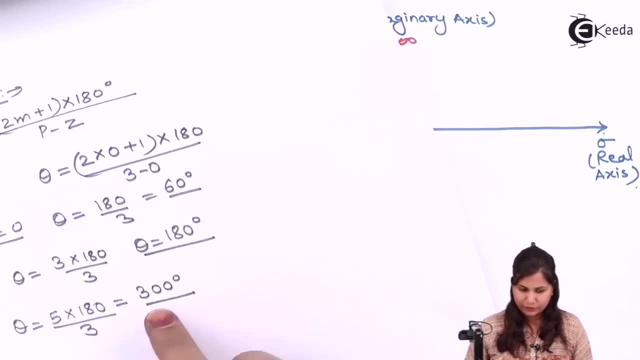 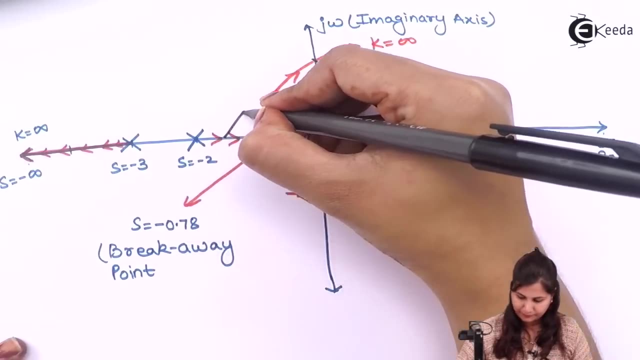 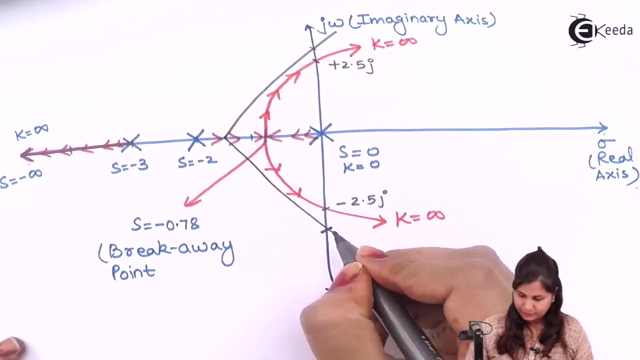 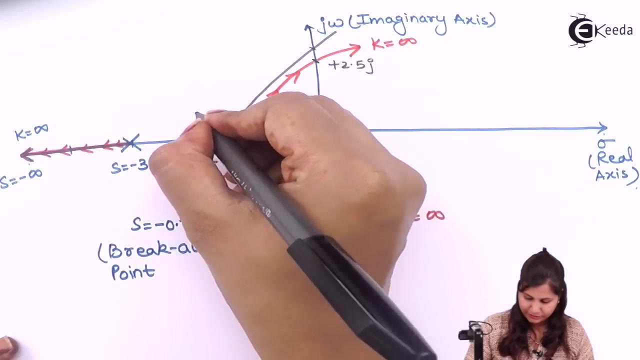 is: this is one of the asymptote, and theta equals to 300 degrees. so from here we are having the asymptotes. okay, this asymptote, this is making an angle 60 degree, this is making an angle 300 degree and one is 180 degree. that is this asymptote and this point.